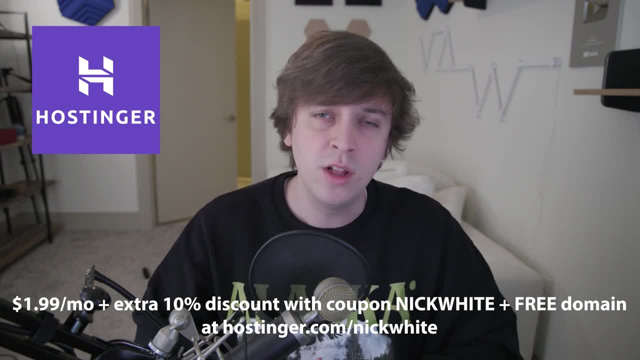 if you click the link in the description or use code NICKWHITE at checkout, you're going to get even further discounts. Okay, so there's a few different ways that we can build a website. The first one is: we're going to build a website, So we're going to build a website. 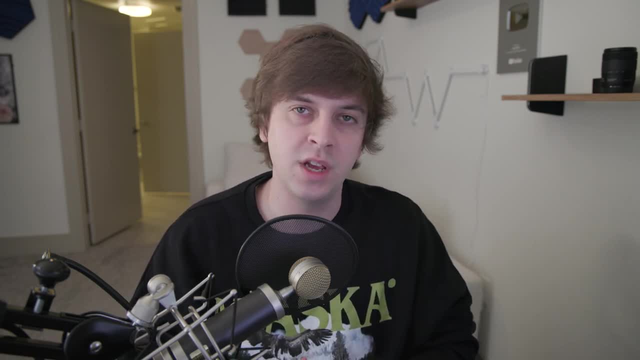 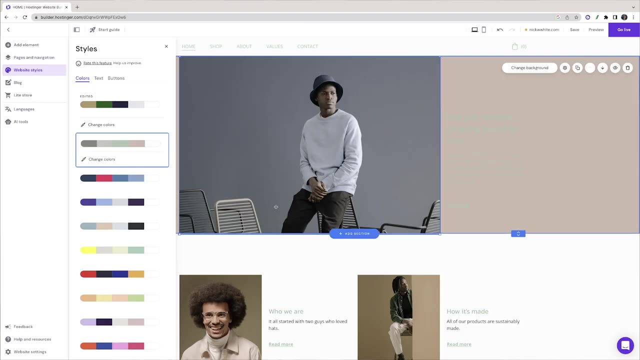 The easiest way is to use a website builder. You may have used something like Squarespace or Wix or Weebly, And this is the easiest way to get a website up and running if you don't know how to code. So you would just go to one of these paid services, you pay and then they have these nice. 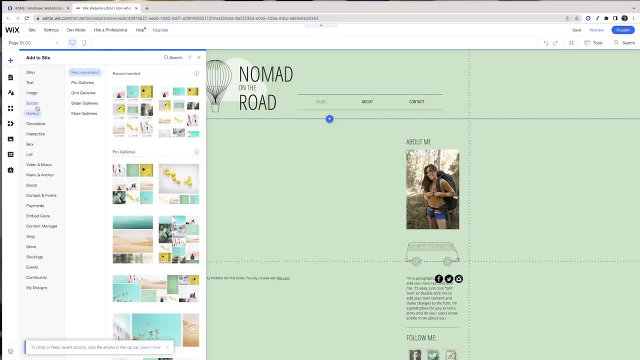 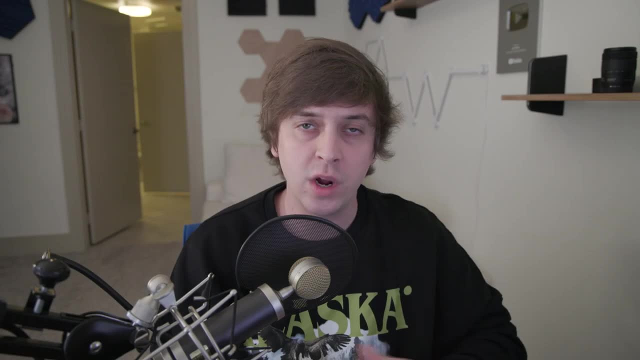 user interfaces where you can drop different user interface components. You can drop text and buttons onto your webpage and instantly publish them and see the live changes. And what's great is that these website builders have come a long way over the years and they're actually pretty. 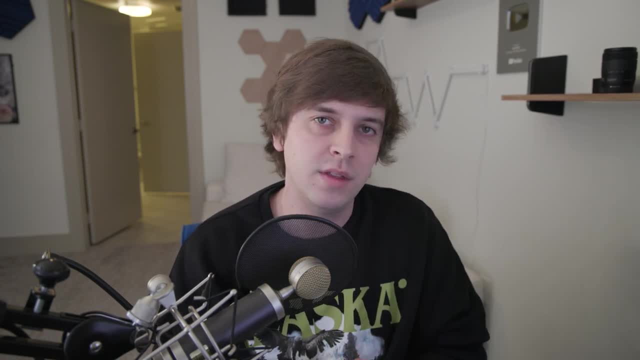 advanced as far as what you can do with customization. However, these are really great for small websites, maybe some small businesses. They do have e-commerce options, So you can set up like payment or just static websites, maybe a basic portfolio, maybe a basic personal website. 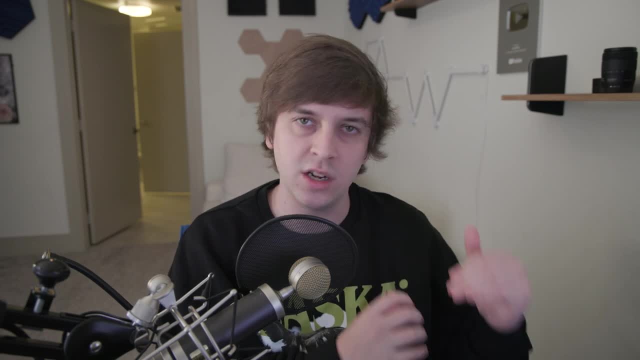 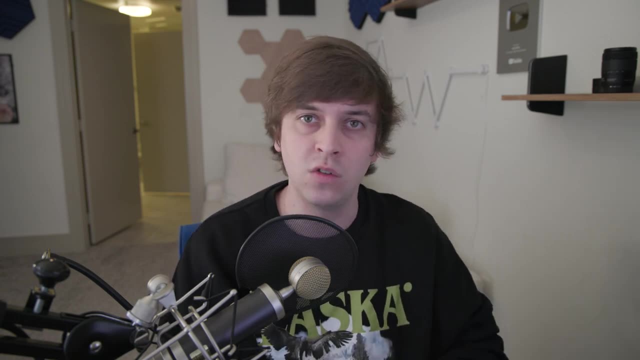 But when it comes to adding a lot of functionality or customization, when it comes to like advanced detailing and the styles and functionality of the website, you're not going to want to use a website builder. Now, speaking of website builders, I'm going to talk a little bit about 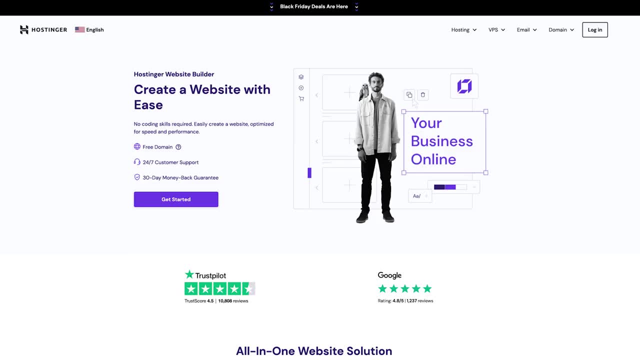 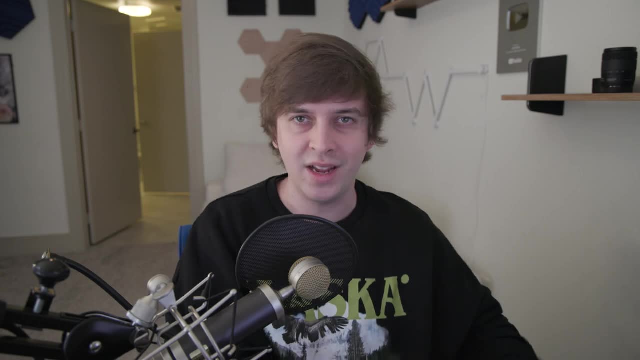 Squarespace, And I'm going to talk a little bit about Squarespace And I'm going to talk a little bit about Hostinger, which is the sponsor of this video, actually has a great website builder that you guys can use if you're not ready to get into coding or other more technically advanced things. 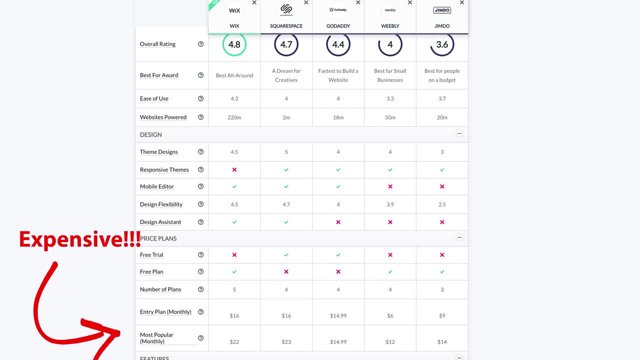 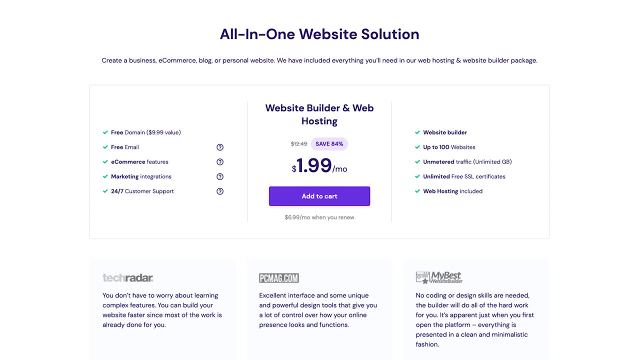 And you should definitely check it out compared to some of these other options, because these options are usually in the $12 to $25 range, whereas Hostinger right now is extremely cheap. If you go into the description and click the link, you're going to be able to get the website builder. 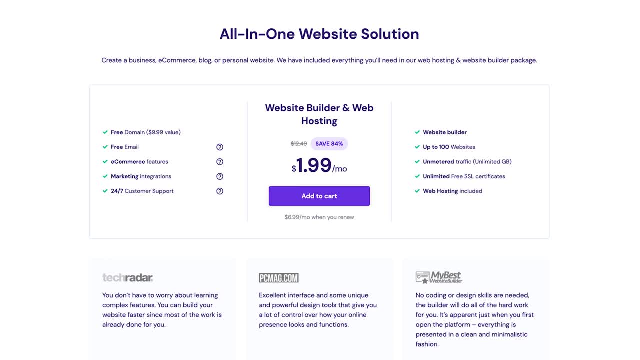 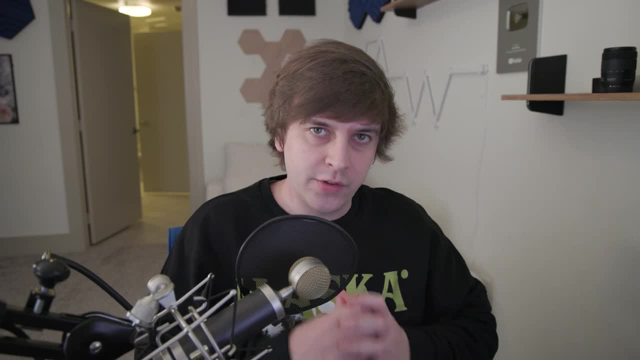 plus much more, for only $1.99 a month, which is way cheaper. And that's even before you enter my discount code, nick white, at checkout for an additional 10 off. now moving on to other ways of building the website, because most of you guys are probably programmers or have some programming. 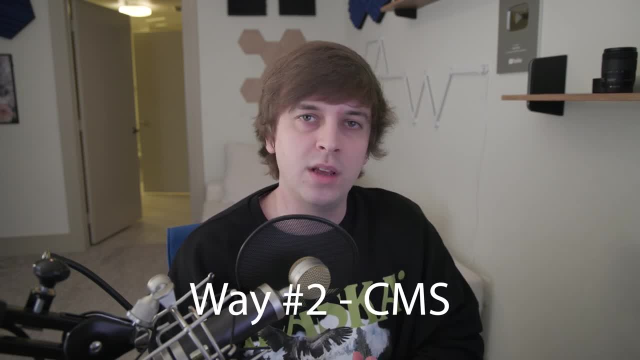 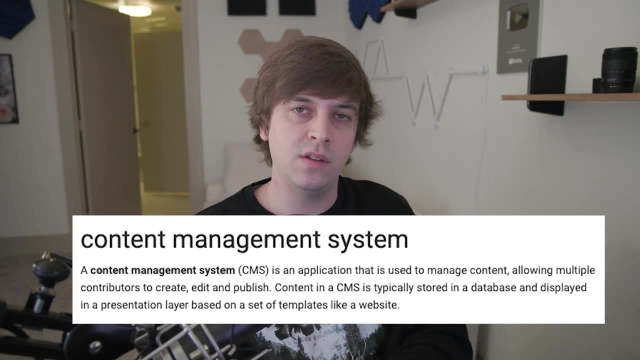 knowledge or experience. so the next way that we can build a website is using cms, and when we think of cms, we're immediately going to think of wordpress. cms stands for content management systems and wordpress is the most popular cms in the world. with a quick google search, we find out. 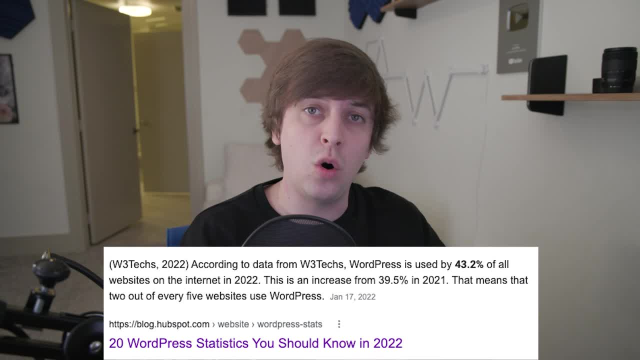 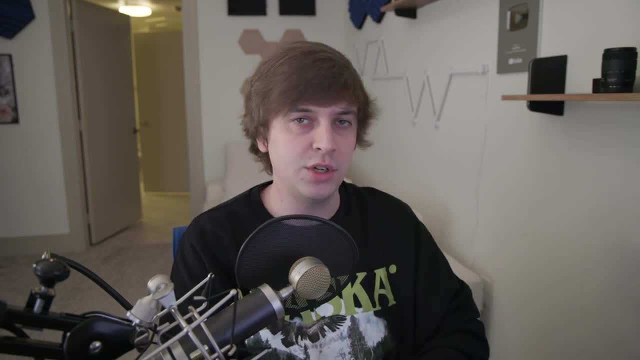 that wordpress is used by 43.2 percent of all websites on the internet. now there's different kinds of content management systems and wordpress isn't your only, and maybe not even the best option, but content management systems in general are great for websites that have a lot of content. 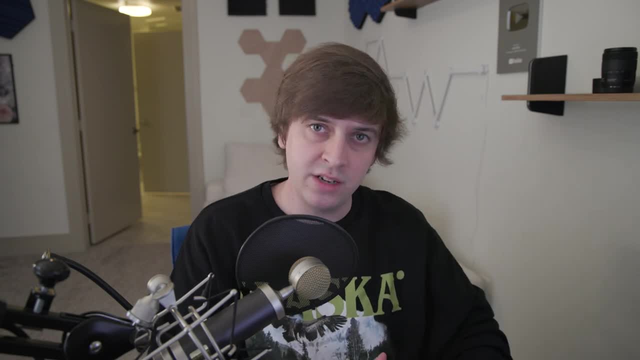 cms is a better option if you're creating large websites with multiple pages or if you plan to make a lot of additional changes to your website down the line. cms makes it easy to do a lot of things like edit pages, add an online store or create web forms. 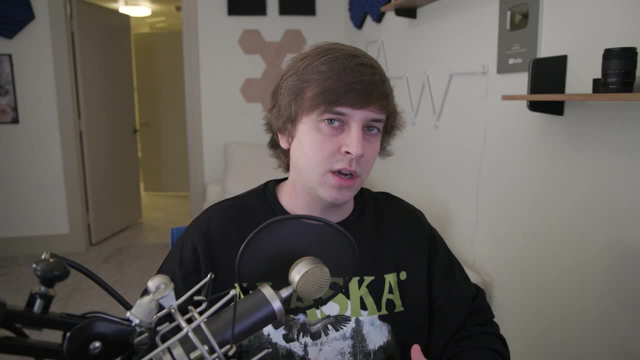 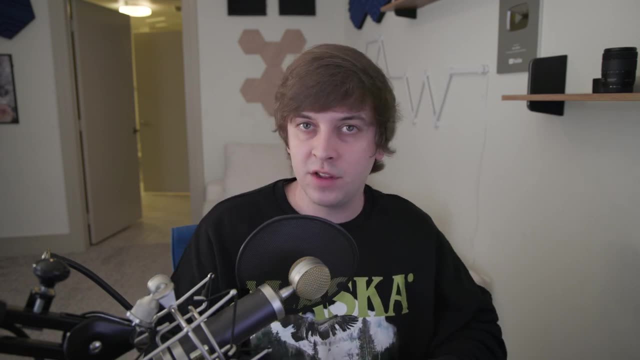 and so forth. so if you're going to be modifying your website a ton and adding a lot of different content, modifying it a lot with different content, cms is the way to go. now, the way cms works is you're going to be working with a content management application, a front end, where you're going to be able to edit the site with a website builder, like user interface. so some aspects from those website builders, but you also can write code and add that additional functionality. so you're going to be able to do a lot with cms that you can't do with a website builder. so if you have a content based website, you're going to want to go with cms. 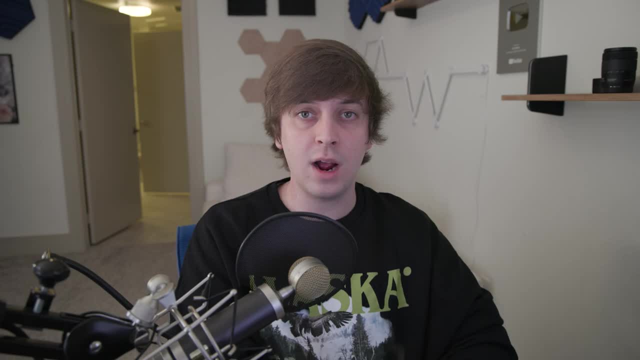 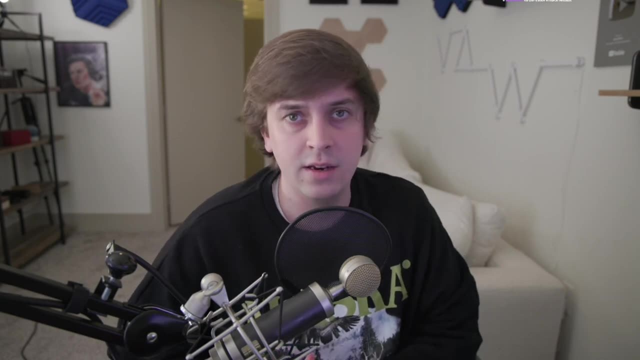 but if not, you could actually code the website from scratch. but before we move on, if you are interested in cms or having a wordpress website because you have a lot of content on the site you want to create, then you should check out hostinger, because hostinger allows you to migrate or build a. 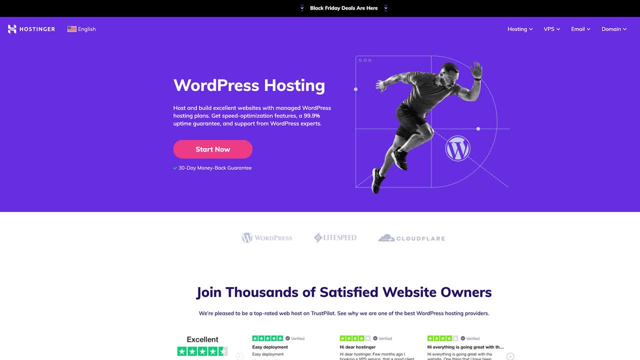 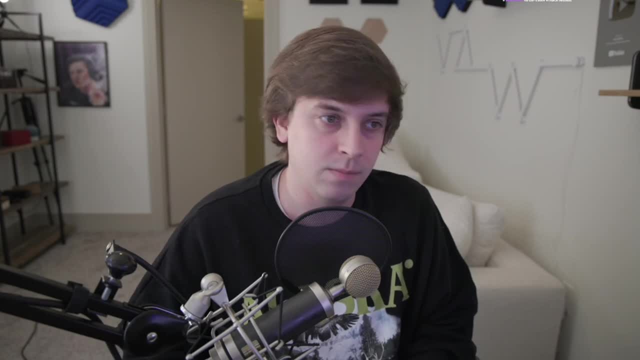 wordpress website and host it on their platform for the low price of two dollars, or 199 in this case, and if you use the code nick white at checkout, you're going to get an even better discount. all right, and now for the third way to build a website, which is my favorite way because 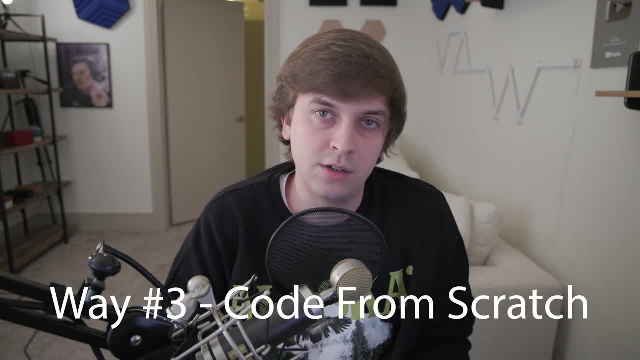 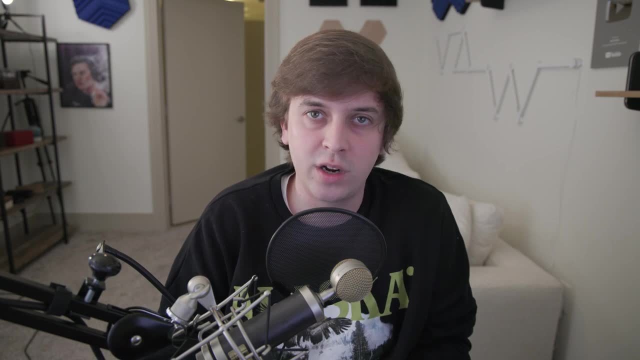 we all are programmers here, and that is to code the website from scratch. now you might have learned other programming languages like python or java, but you don't necessarily know web development. so i'm going to take you through a very quick web development tutorial. so at a basic level to build. 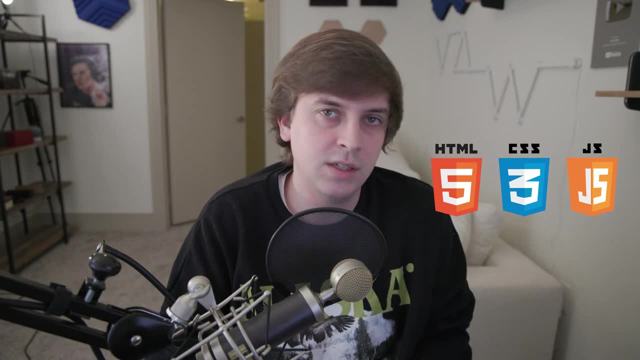 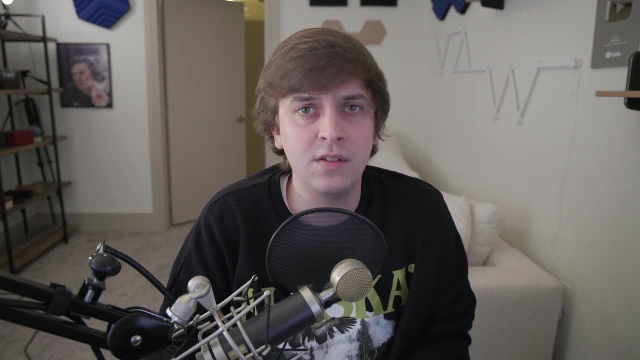 a website. you're just going to need three different things. you're going to need html, css and javascript. html stands for hypertext markup language. you're going to be coding in a markup language. it's extremely easy to learn and this is going to be the skeleton. 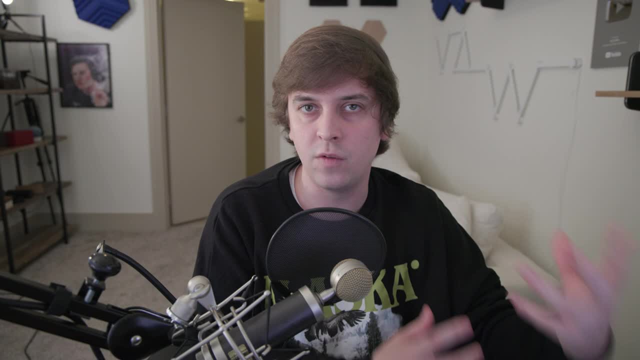 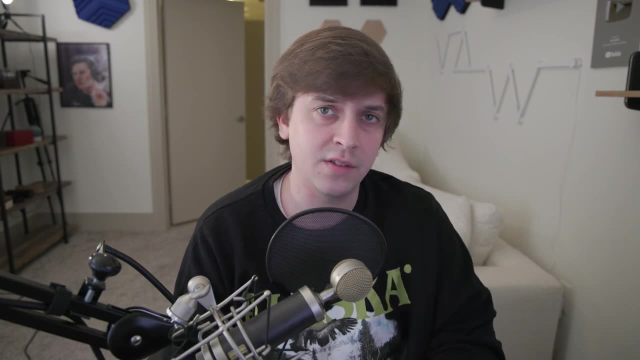 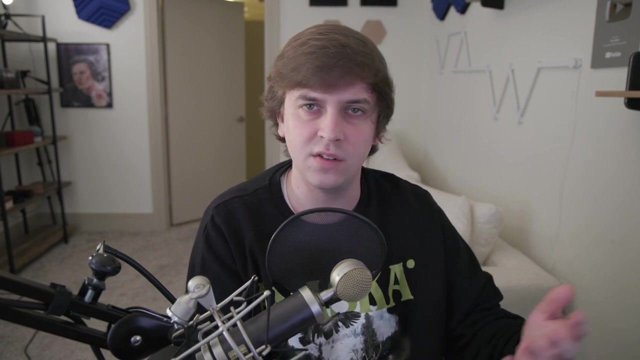 or the actual content of your website. no styles, no functionality, but actually just the content, for example, text or buttons or images. css stands for cascading style sheets and this is going to be all the styles for your website. so the text, the decorations, font sizes, the font colors, the color. 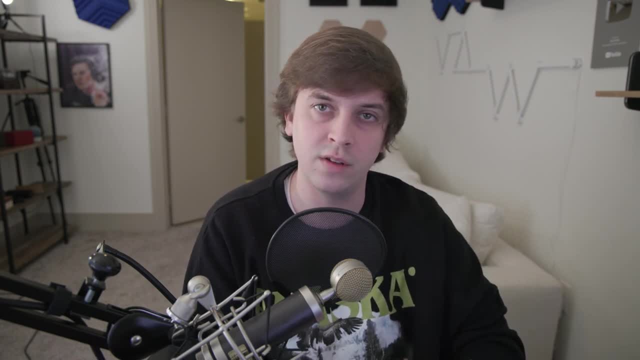 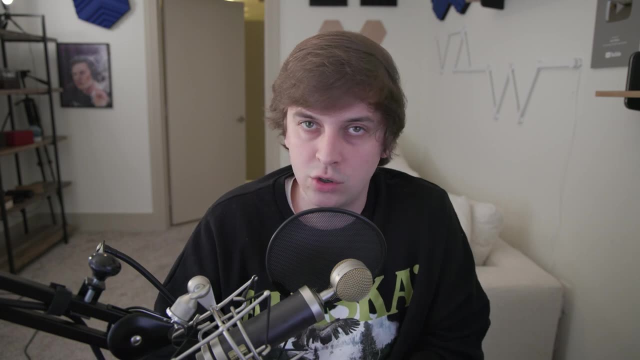 the background color. all of this stuff is coded in css and you're gonna have full control over how your website looks using css. and then, last but not least, we have a javascript which is more like your own personal programming language. we could do object oriented programming. there's no classes. 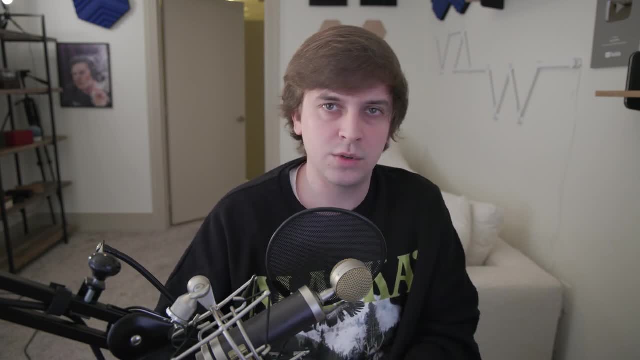 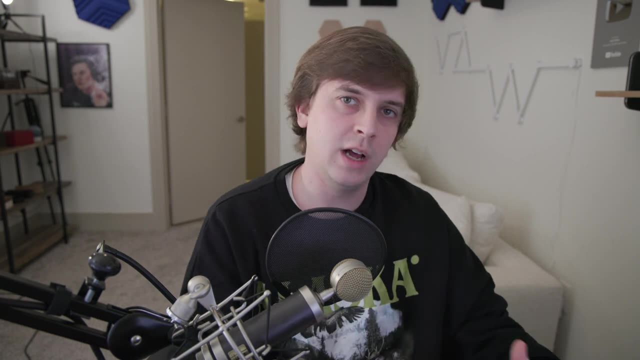 but it's a lot like python or java or something like that. javascript's going to come into play when you have things on your website that do things right. so if you have a button that does something when we click, we'll have javascript execute in the background, so a function will. 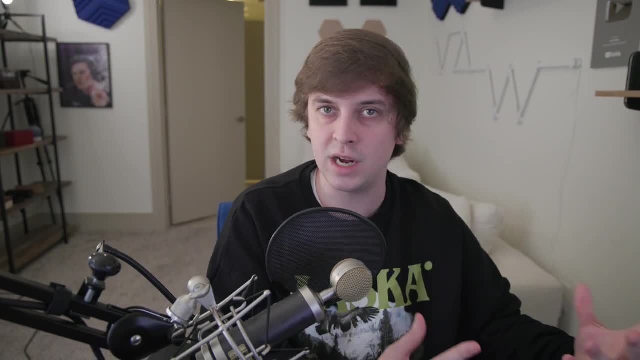 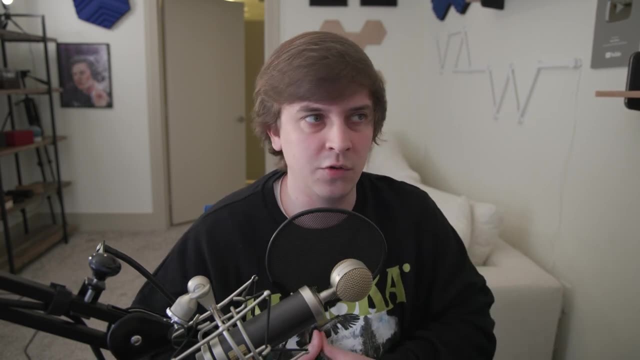 execute. maybe it does something like alert. a little alert box will pop up saying hello world. anyways, i think we get the general idea for that. so all you'd want to do is just make three different files. one is going to be indexhtml, one of the other three is going to be indexhtml, one of 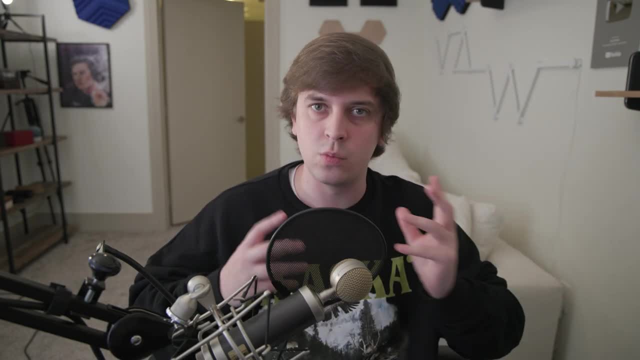 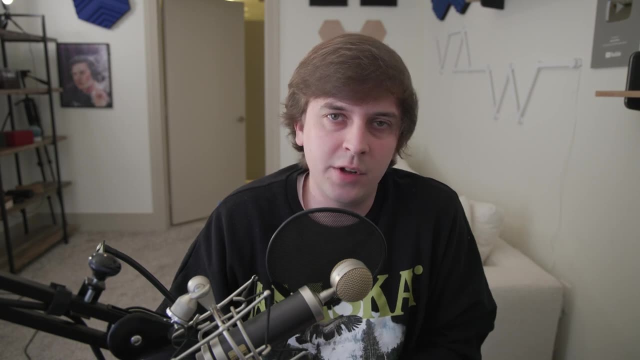 the other three is going to be appcss, one's going to be appjs, and these are those three languages respectfully. so you need three files only to build a website, and if we open up those files, we get started coding immediately. if you're not familiar with html and css, you might want to. 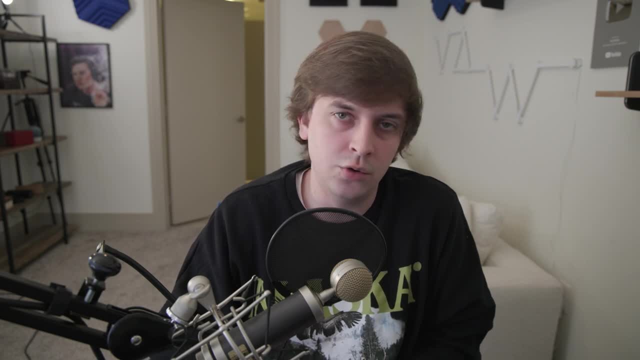 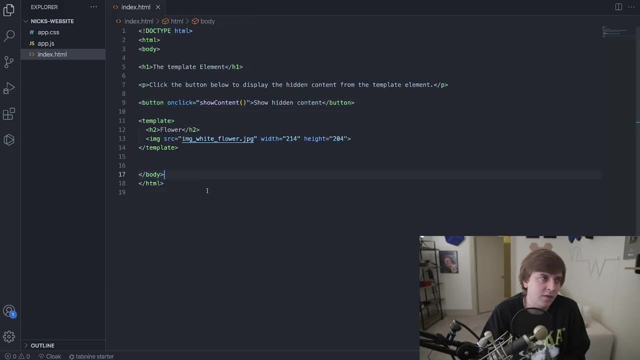 go through a code academy tutorial or something like w3 schools or tutorials point. do a quick tutorial. you should be able to pick these up in about an hour, but basically you just want to look up the template html code. this is how the standard html looks, for every website, html is made up of. 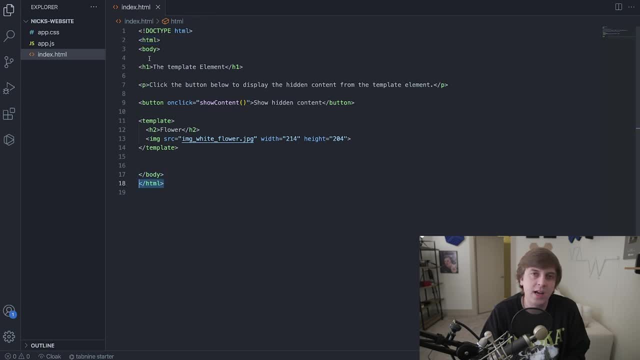 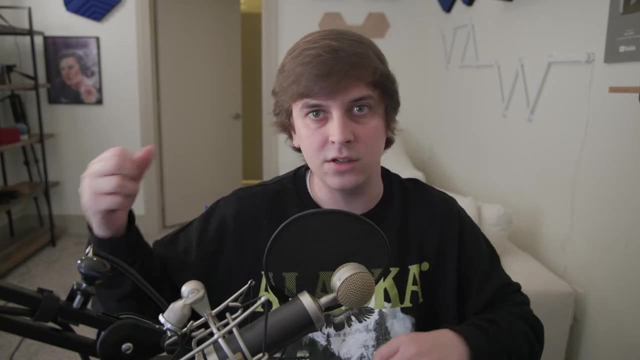 tags and everything's wrapped in the html code. so if you want to look up the template html code, this is how the template html code is made up of html tags and then you have a head and a body. i'd consider the html the root of the website, and then it hooks up to your other files to add the styles. 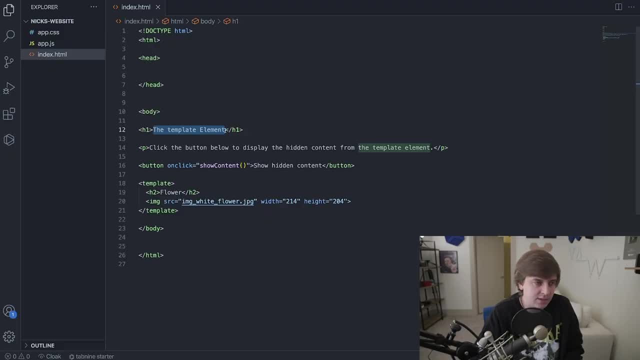 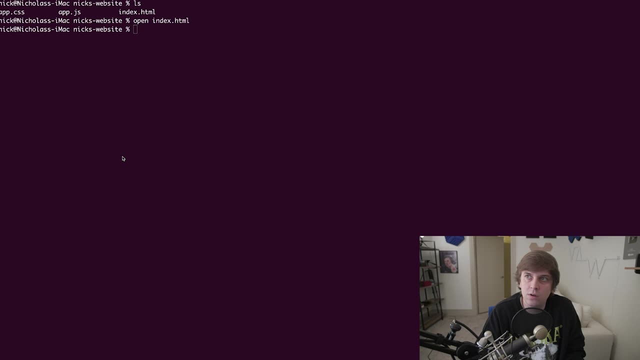 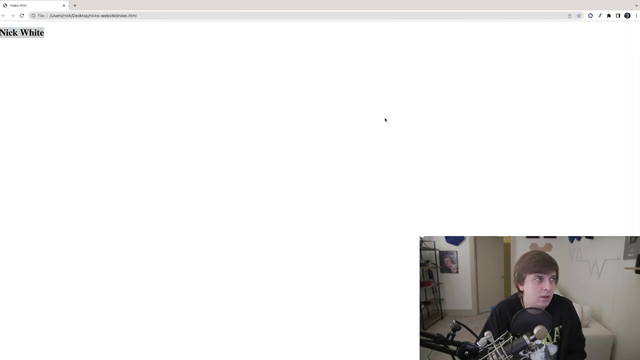 to add the functionality. if we look, we have some h1 tags and that is a header tag, so i could put my name and this will be a header on the website if i were to simply open up my indexhtml. now we have just nick white. if we wanted to add a button and i said, click me for the text of the button. 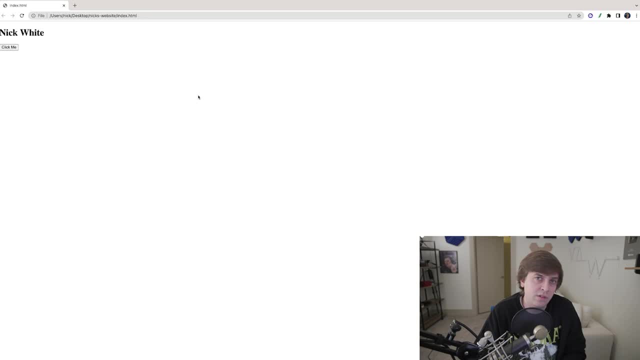 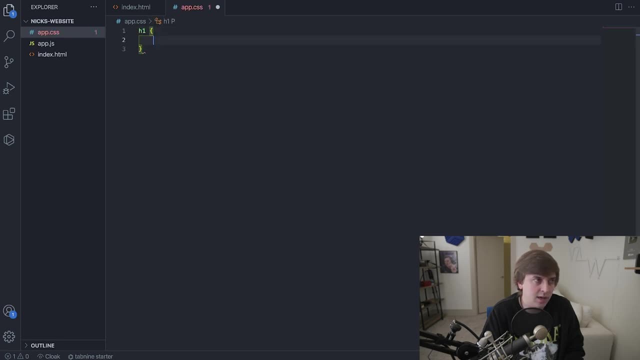 we'd go back to the website and we'd have click me. notice how the button doesn't do anything. now, if we wanted to add some styles to the website, we'd go into our css and we would target the h1 tag. so you target a selector and add property value pairs. so we're going to do. 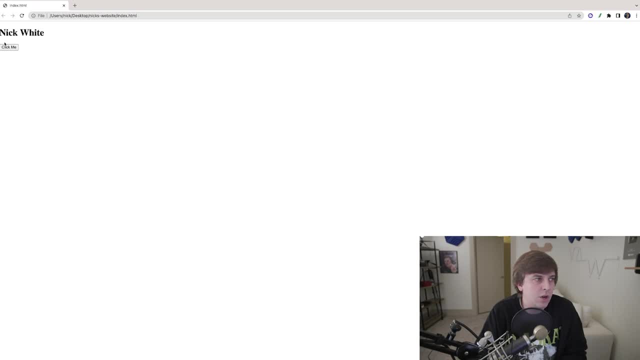 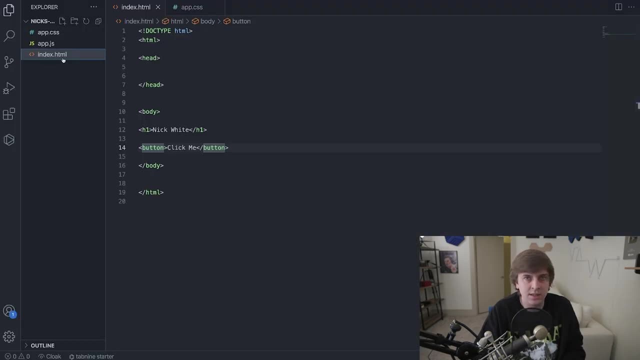 color red for the title and if we go to our website and we refresh, it's obviously not going to be red because the css isn't hooked up to the html. so you actually have to hook the file appcss up to our html. that's going to be in the head. so right here i have the link tag in the head. 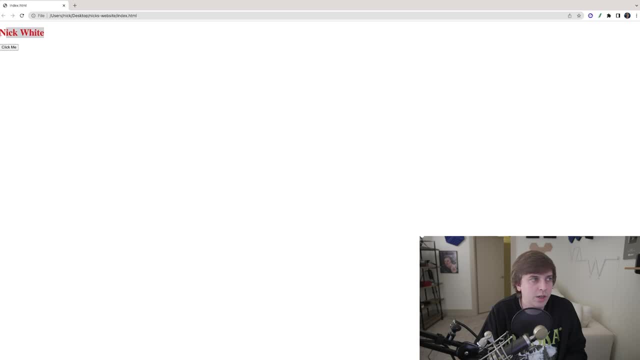 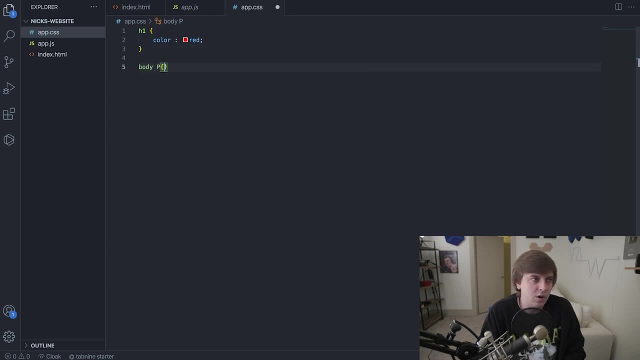 and you can see the link is appcss. we go over here and we refresh and now the colors and styles will take into effect. there's a million different styles you could add. so, for example, if we just wanted to target the entire body of the website, which is basically the whole website, and we wanted 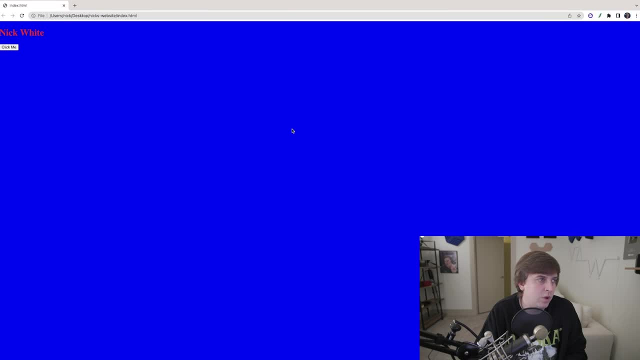 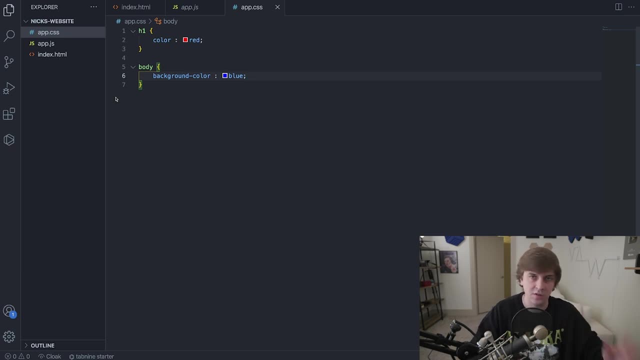 to do background color and then we wanted to do blue. we could go to our website and then the background color is blue. so you can look up all the properties and values for css to figure out all the designs and things you can do by yourself. you can do animation, you can do all these crazy. 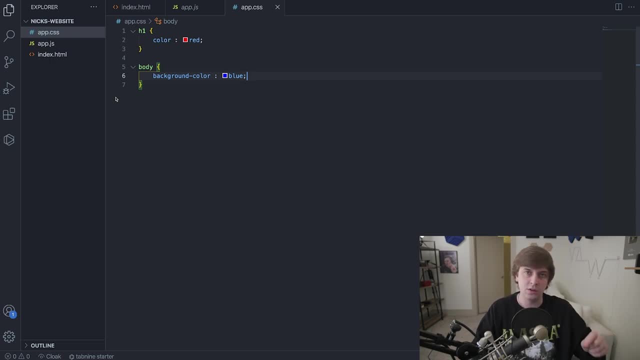 things, uh, down to the very smallest detail. so that's why coding is great, because we have full control over every single thing on our website. now, last but not least, we have javascript. so javascript, we actually can write code like real code. so let's say, alert button is a function that we're going to make, and then let's just call alert. 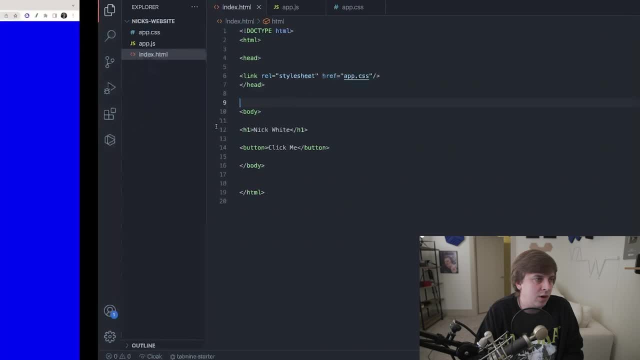 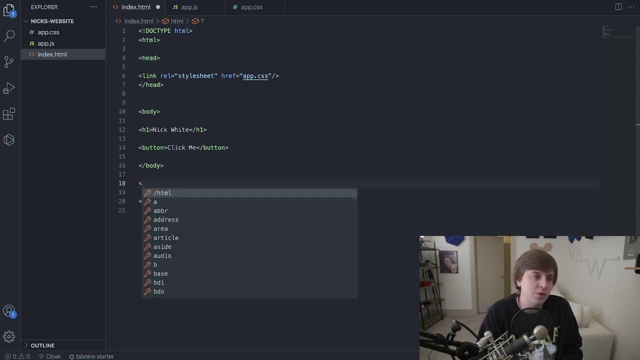 hello world, and now we would just have to link it right. so if we go to our website and i click the button, it does nothing still. but if we link this- and with javascript, i'm usually going to add the link at the bottom because i still want the page to load with. 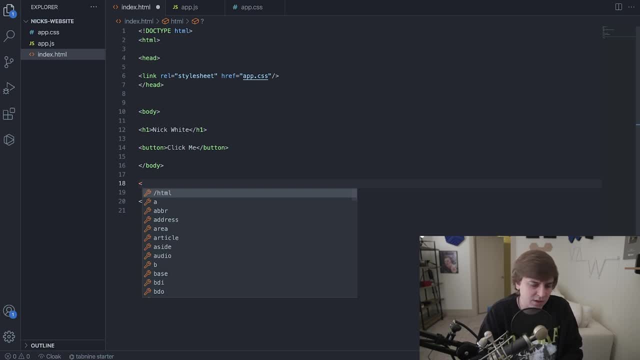 the content and styles, even if there's no functionality because something gets messed up. so i'm going to do script and then we do source equals appjs. and there we go, it is linked up to our appjs. we go here, we click. however, this still isn't going to work, even though we linked. 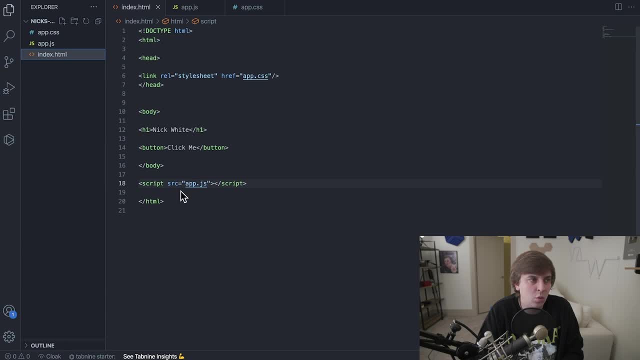 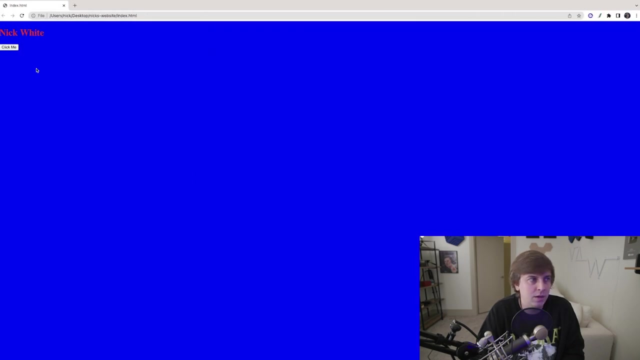 up the javascript file and that is because we're not calling the function. so once we're linked up we can actually use those functions from the javascript file. so we're going to do on click equals and we'll do quotes and we will alert button. we'll call alert button. now we go back. 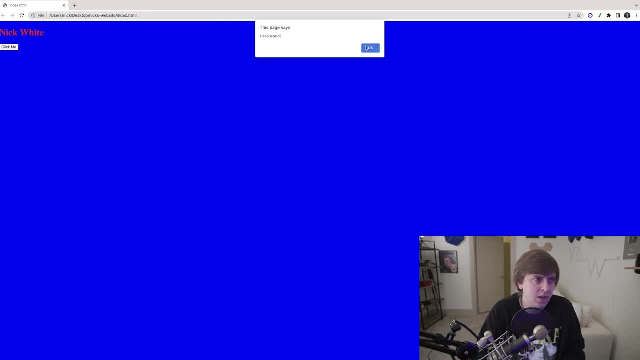 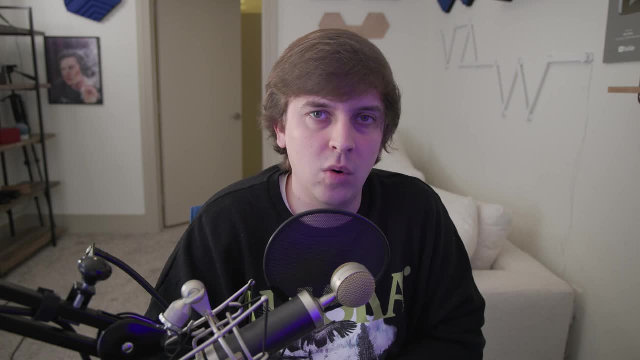 we click and the function gets executed from javascript. we get hello world. so this is my crazy website that i built in a few seconds, just giving you guys kind of a demo. but now i'm going to show you guys how you can deploy this, whether it's for to free hosting or to a paid hosting. 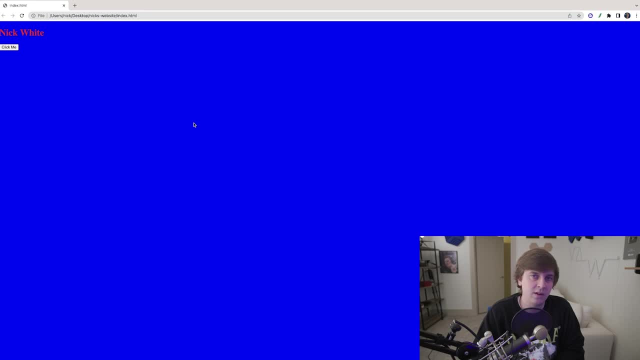 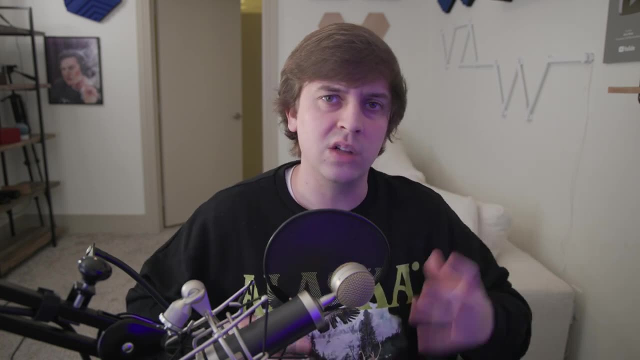 platform and this would be your website. that's how easy it is to make a website. of course, you'd want to to look a lot better than this, and i'm going to tell you how to do that as well, like get a website up and running really quickly using code, but i'm going to show you how to host this. so there's two. 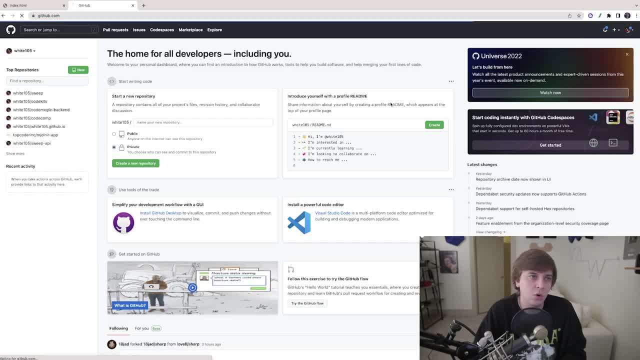 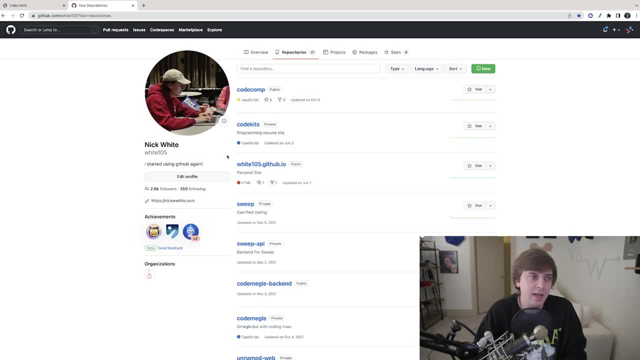 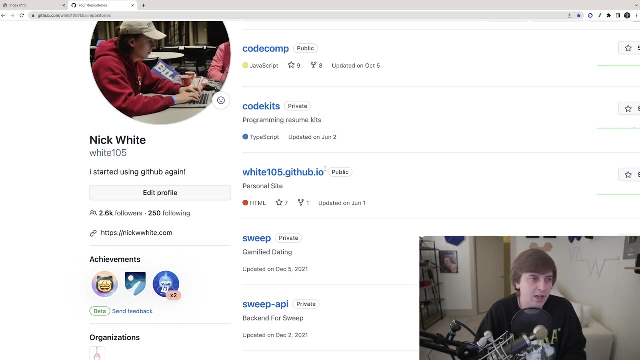 ways i'd recommend to host a website, one of which is through github pages, which basically you can make a repository, so a folder for your website on github, and you're going to want to use your usernamegithubio so you can see here, my username is white105.githubio. this is a personal website. 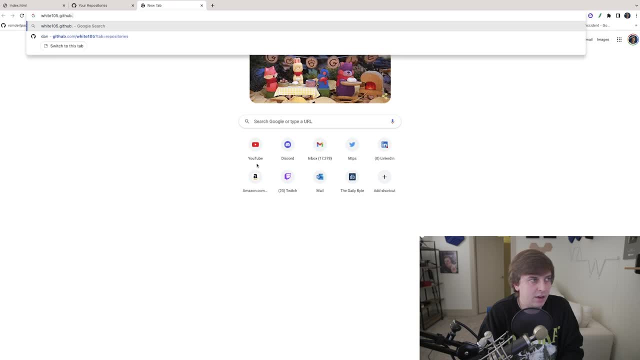 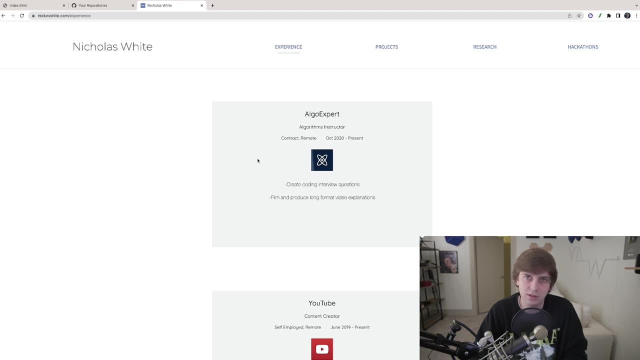 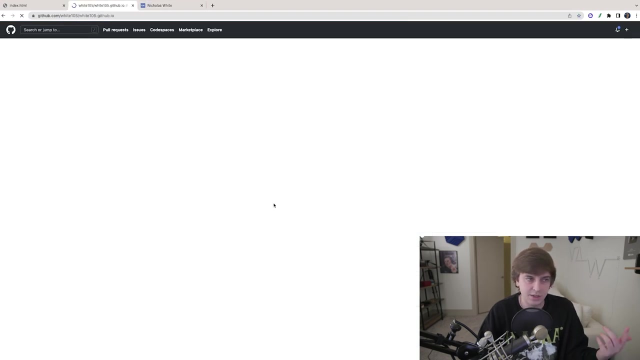 and if i were to go to white105.githubio, this would be my website, and this is completely free hosting for static websites, basically. so if there's not a lot of functionality going on your website, github will host your site for free. you make a repo, it's just going to take your indexhtml. 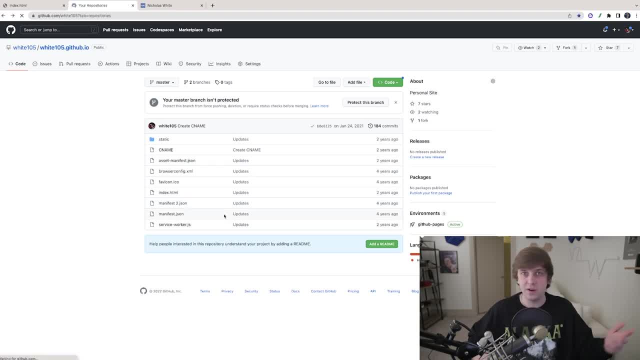 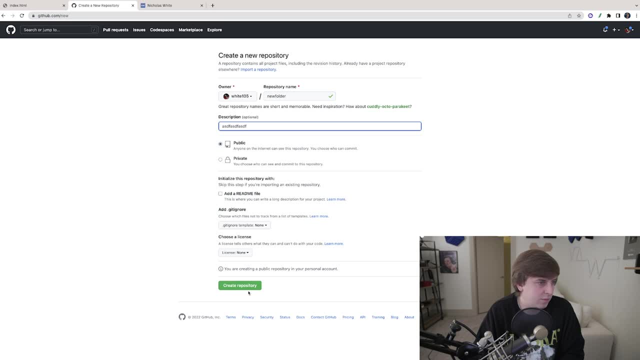 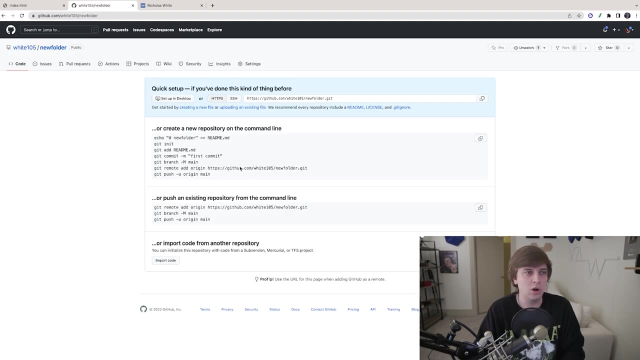 from when you commit the code and it's pretty straightforward. it's pretty awesome and if you really want to walk through this, all you do is like new folder, right, you would make a description. you know you could add whatever you create the repository now you could follow along with these. 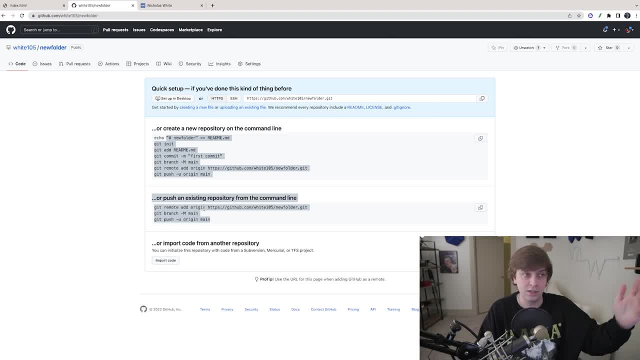 steps: to use git to push your code up. so the html, css and javascript. you just push it up with git, or you can literally just import it. you click the import button and drop your code in. so the folder of files, the html, css, javascript. drop it in with the import button. you know, refresh, boom. 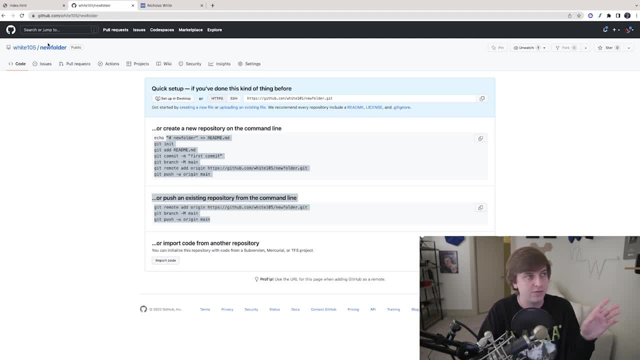 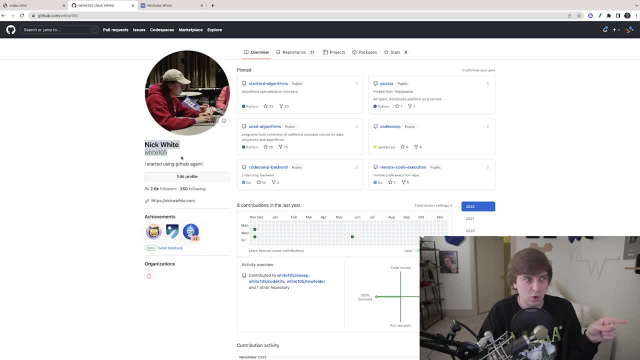 your website is up and running right, so just do user. you just have to name the folder username, so your user name, and then you just have to name the folder username, so your username, and then you just have to name the folder username on github dot githubio, so white105.githubio or your. 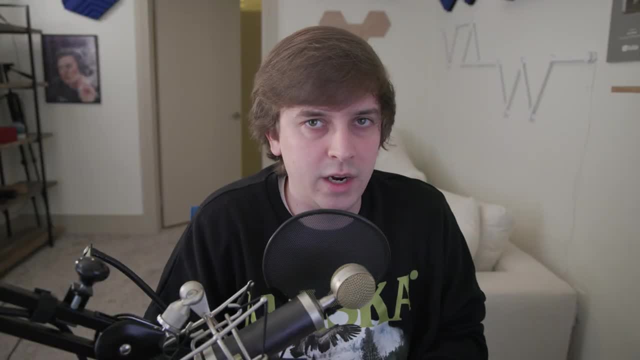 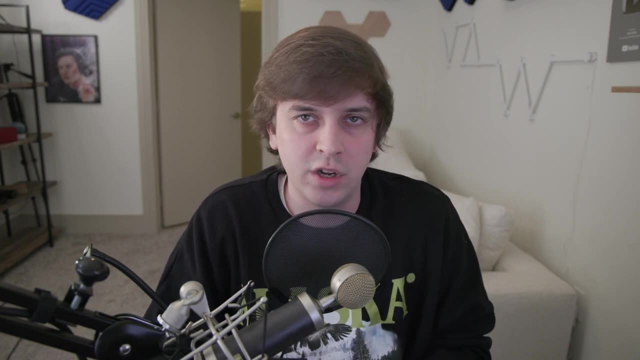 usernamegithubio. so now this has limitations, though. right, if you have a back end, if you have an api, if you have a database, if you have anything uh special going on on your website at all github pages isn't really going to work. so it really only works for static websites, and in that case, 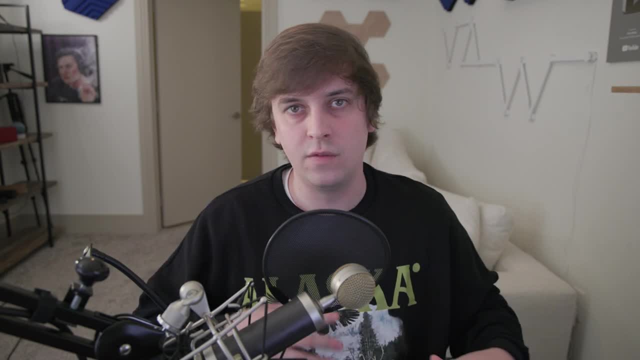 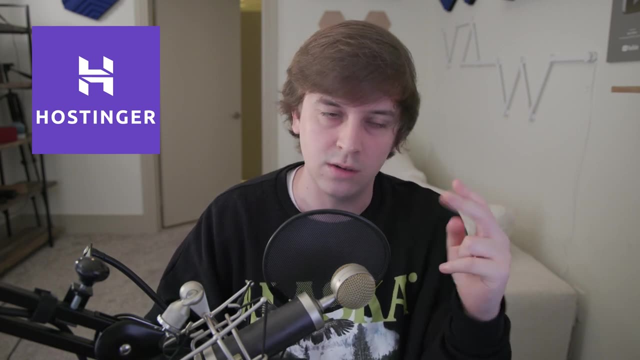 you're going to want to head over to get paid hosting, which. there's a variety of options. however, one of the cheapest and one of the most high quality ones is the sponsor of today's video, which is hostinger, and with hostinger guys, this is amazing deal going on right now. go into. 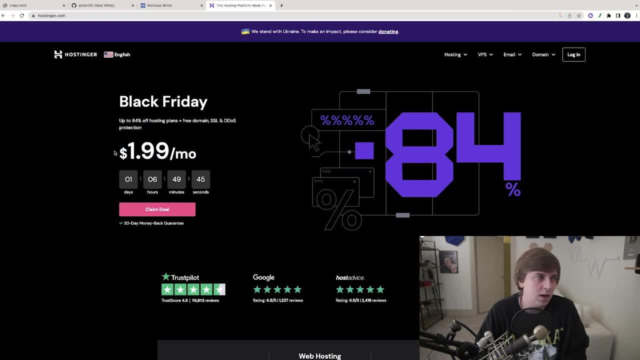 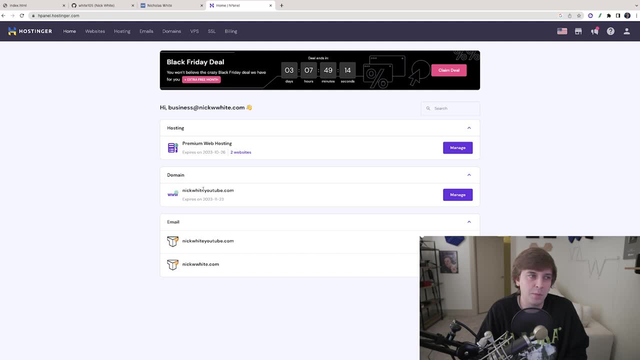 the description, it's 199 a month. this is amazing. uh, use my code, nick white, at checkout and you get even further discounts. and when you sign up for this premium hosting, you're also going to get a domain, which is expensive on its own. you're going to get a free email. you're going to get up to 100. 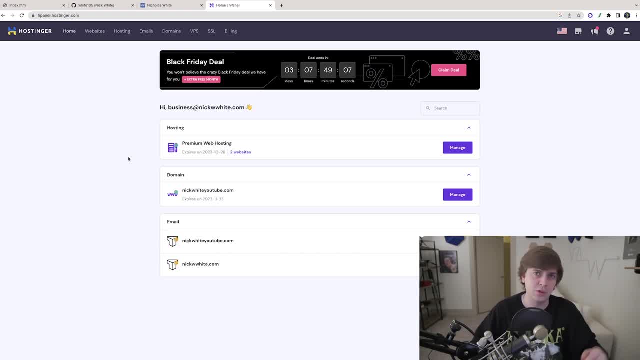 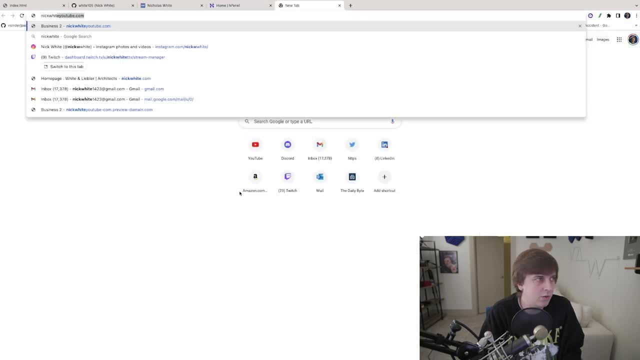 websites. you're going to get a variety of features that are really valuable for two bucks a month. so i made a new website yesterday with a free domain they gave me. this is nickwhiteyoutubecom. if we go to nickwhiteyoutubecom right now we could see it's just random template code that i dumped into it, but i'm going to show. 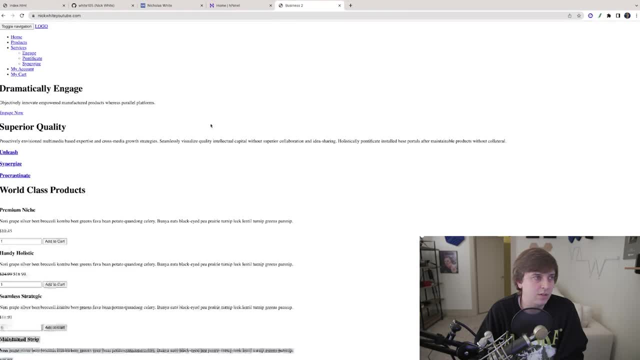 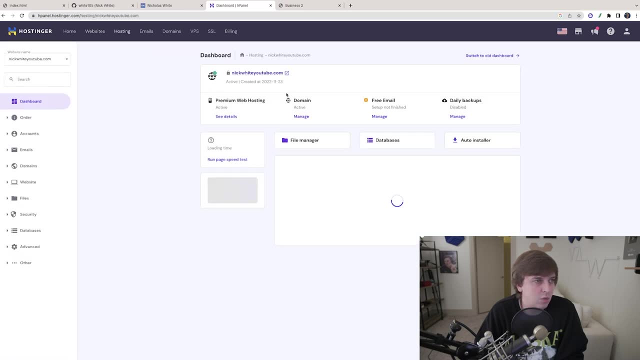 you. this is the website i just made in front of you in a few minutes, and i'm going to dump this and show you how easy it is to get this up and running on nickwhiteyoutubecom. so here we are with my websites. i'm going to go over to manage nickwhiteyoutubecom. i'm going to go to file. 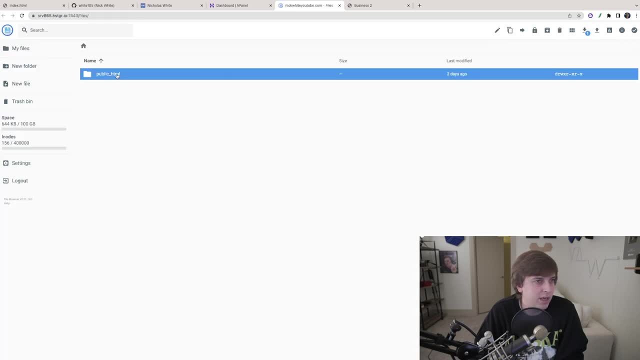 manager and now we're in hosting as file manager. you can see public html and this is all i have in here right now, just one html file. i'm going to delete this and then there's going to be nothing on my website, and then from here, it's super easy: just go up here to this little upload button. i'm 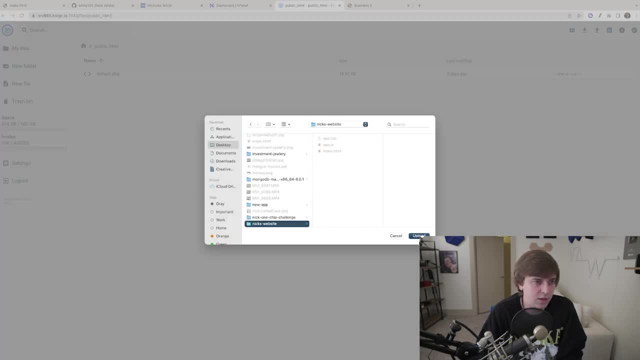 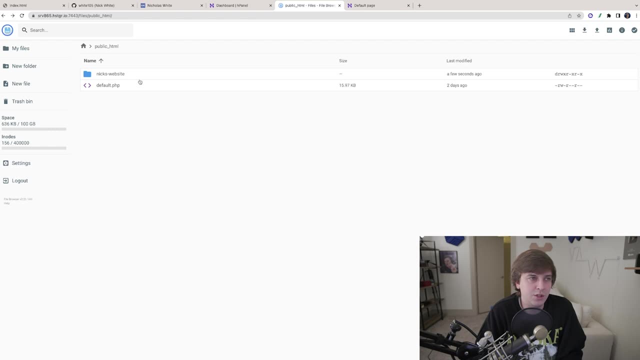 going to go to click folder, because that's what we did: nick's website. i'm going to upload this folder. so boom, website's uploaded now. i do want to distinguish that you can't just dump the entire folder and then hope for it to work right. the website's down right now, but you have to extract. 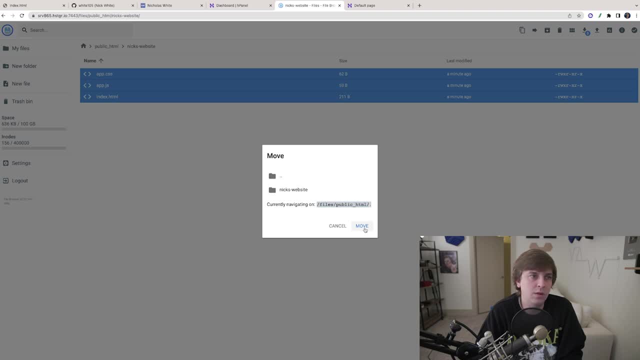 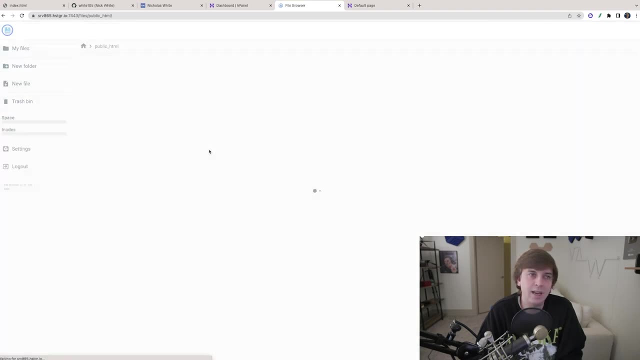 the files from this folder. so we're going to move the files one little step back. we're going to just move these and then we're going to get rid of the folder. we don't even need it now. we're going to get rid of the folder and then boom, now we should be good to go. so you just want all of those files. 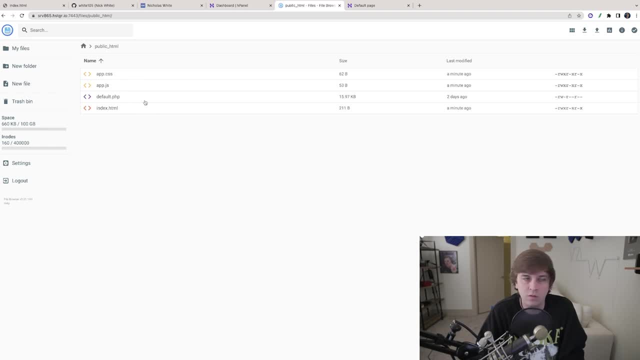 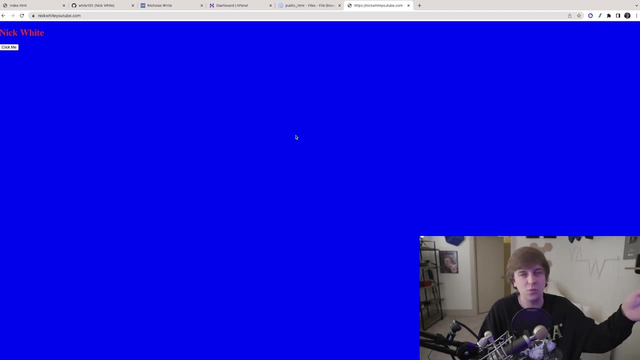 i mean you could just drag and drop all the files instead of the whole folder. but i just wanted to show you because i think some people might be confused about that. and now when we go to my website you can see. this is the website i built for you guys. in just a few minutes it's already. 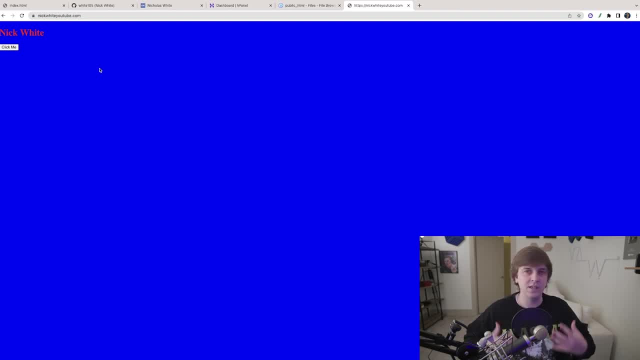 up. i mean, that was instant. so, nickwhiteyoutubecom, my website is already up now. i will say it's extremely ugly. so how would we get a cool looking portfolio website up and running using code? well, that's where you're going to want to go, to bootstrap templates, right this? 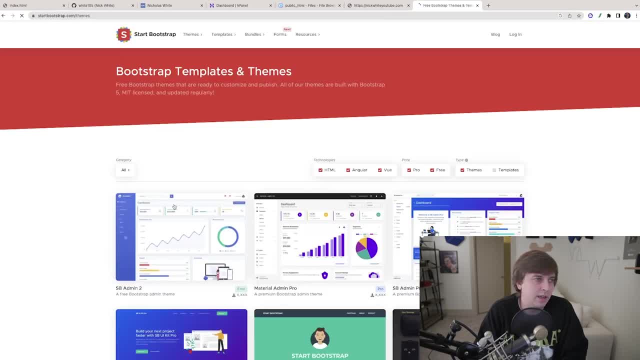 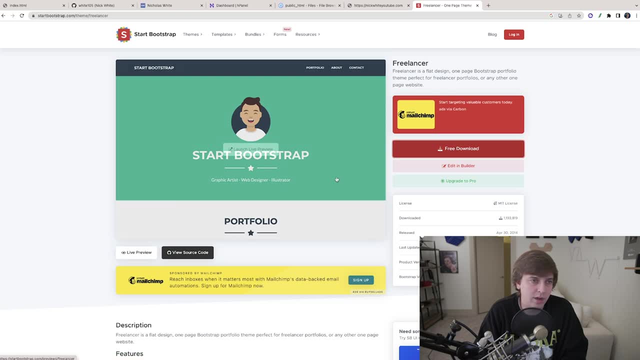 is, if you're short on time, uh, if you just want to like get a bunch of template code to start with, you could easily just go over here, look. so here's a website we can launch for live preview. we can get a free download of it, and so we just downloaded this bootstrap template, which took like two seconds. 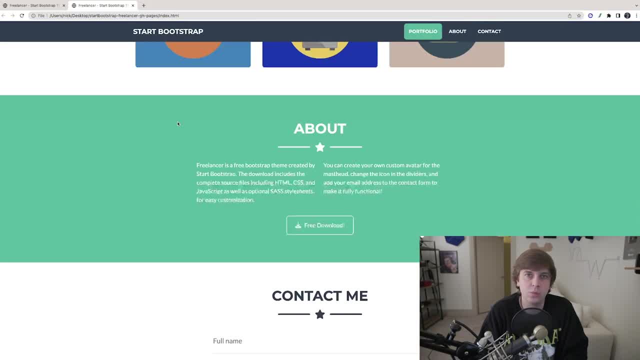 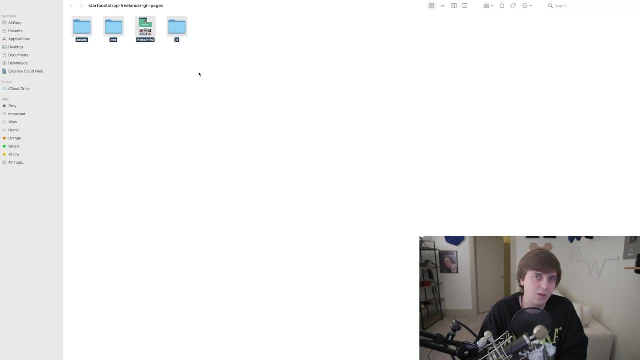 and i opened the html and look, we have this whole static website that we could start with. and this comes with all of the code, right? so i could just dump this, all this code, into hostinger and let me show you once again how simple this is. so let's just go over these files. 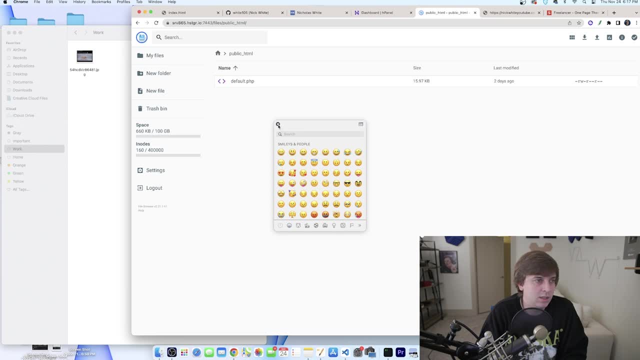 these are the ones we added for our website so far. i'm going to delete these. so we have nothing on our website and it's instant refresh every time. so if we go here, look, the website's gone now. now let's just drag all of the stuff from our bootstrap template we just downloaded, right? so this is the. 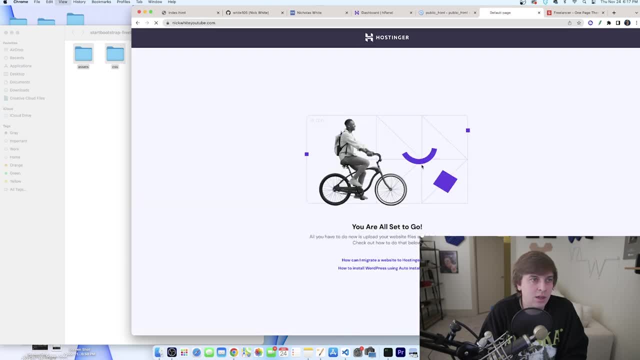 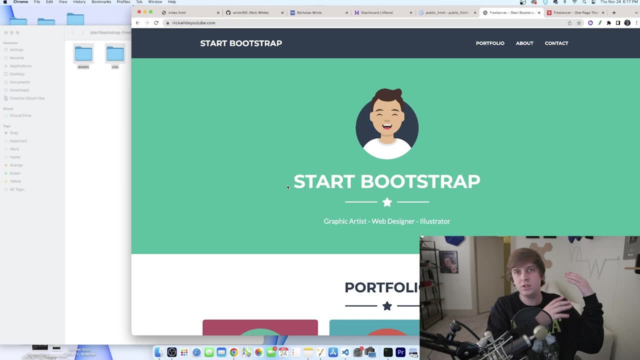 bootstrap template, we could see we have the index html in the right place and if we go over to our instant refresh, this is live. you guys can go to this right now. so that's a whole template website. we got up and running in just a few seconds and now we could easily modify this website, right? i? 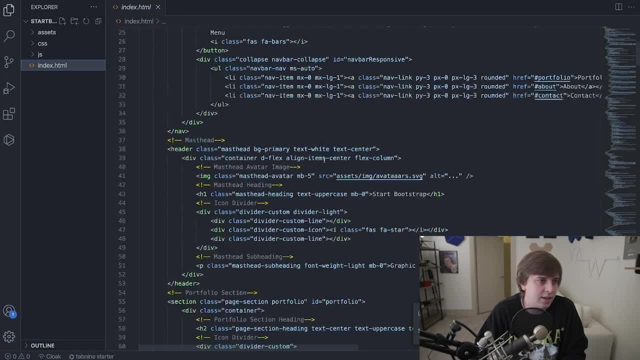 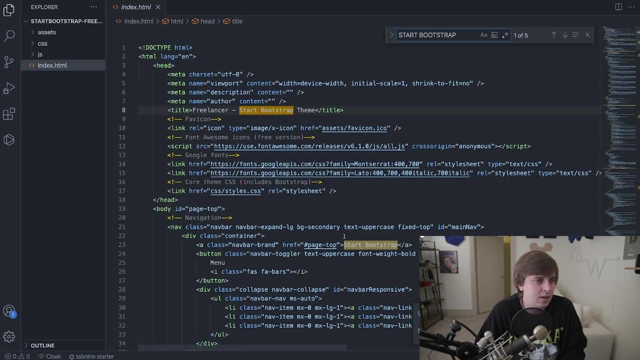 just pull it up in my text editor. we go over to indexhtml and we just start editing. so let's find start bootstrap and replace our name. so here's start bootstrap. we're going to go down here. we could say nick white's website. so here's nick white's website. so here's nick white's. 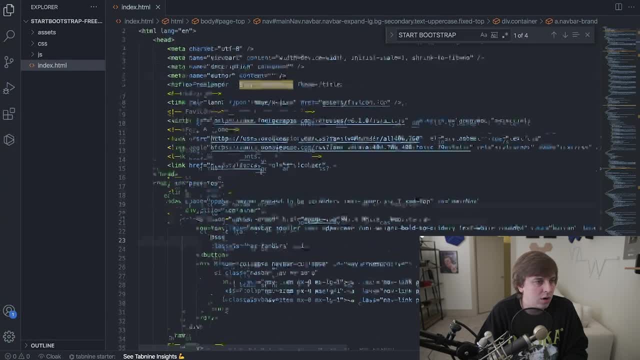 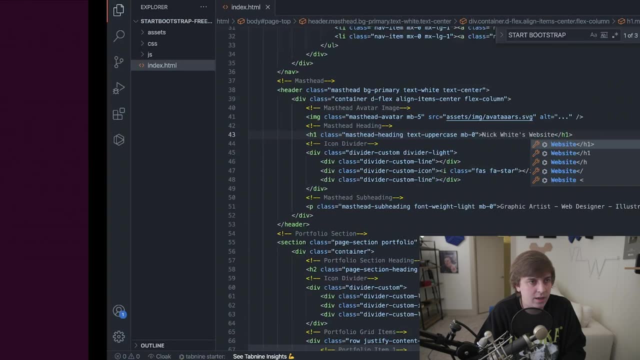 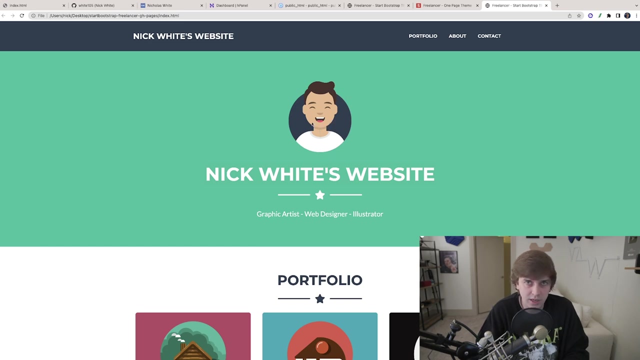 website. you could see this updating. we go over to our code, we're going to feed our start bootstrap again. we'll say nick white's website again, and we're already getting a portfolio up and running. right, i'd replace this picture with a picture of me. and so the last thing. 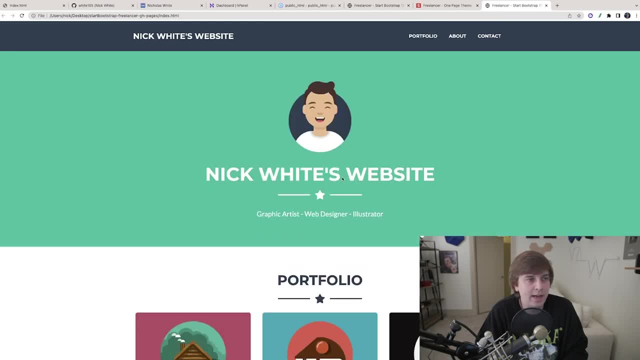 when it comes to coding a website, i do want to mention is when you're editing the website on your local machine, that is not going to update on the official website automatically, right? so this is still the official website. nick white's youtube: it still says start bootstrap, even though. 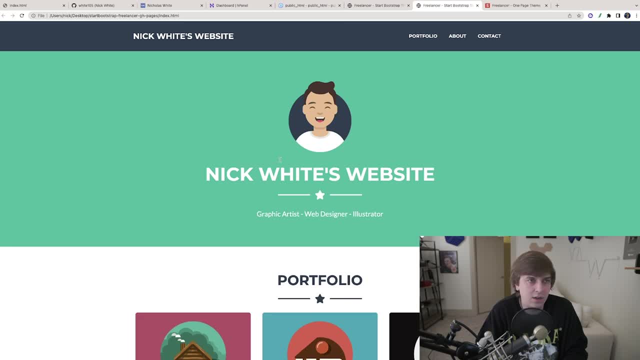 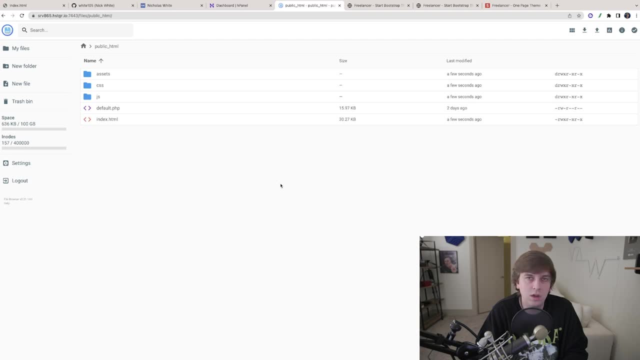 i've been editing it and this is on my local machine. this is the code, so what you're going to want to do is just make sure you have the updated version of each of these files in the public html on hostinger. so this html is outdated, so what i'd want to do is just delete it and re-add the. 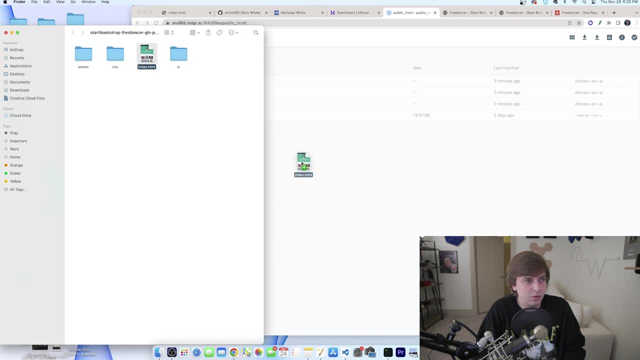 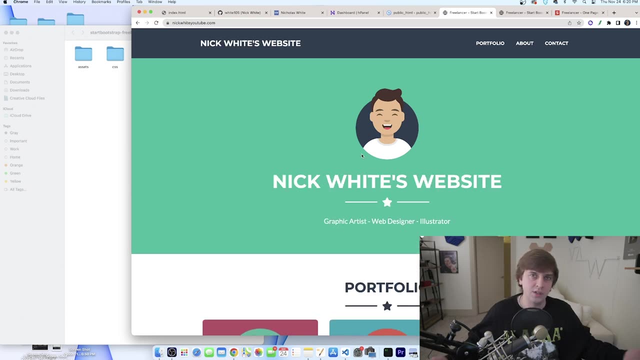 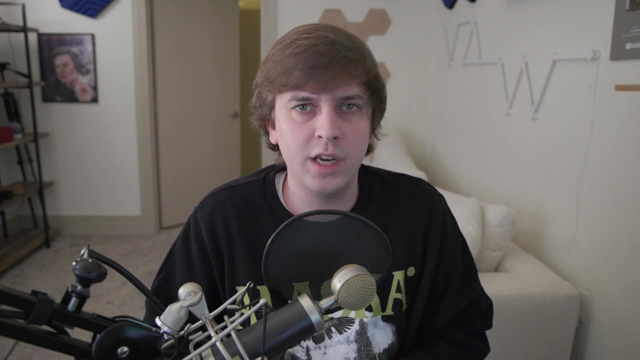 updated html file, and so here's the updated file on our local machine. i drag it in. it's an instant update. so we go to our actual website, and there's nick white's website being updated now. if you're comfortable with web development or just don't have knowledge of html, css and javascript, then you probably don't even need. 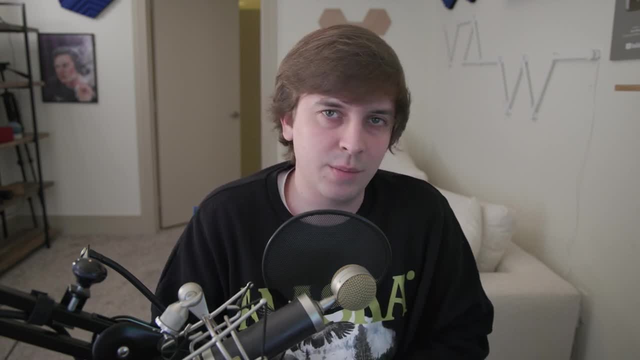 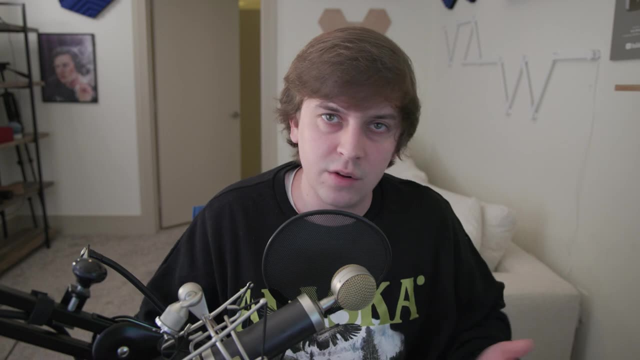 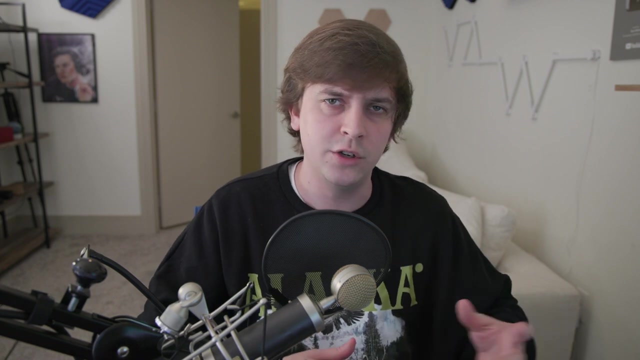 bootstrap, you could code this all from scratch, and when it comes to that, i highly recommend looking up some of the upcoming top coders in the industry- maybe consulting companies. look up, look at other people's portfolio websites. get a feel for how people are designing their websites. what looks good, what user interface looks cool to you, and then start to code your own. 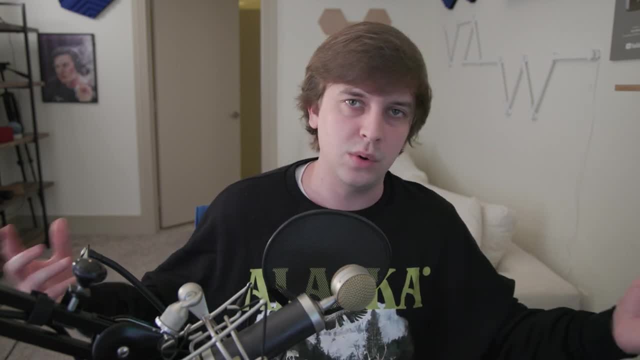 website down there. so there's all the different ways that we can do it, but we've done a lot of it, and so i would recommend trying this out for yourself, and i think it's a great exercise. to just try it out for yourself and you'll see if you like what you've learned. it's free, it's easy. 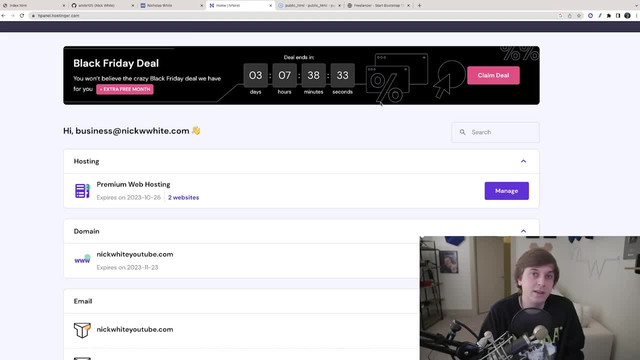 to create your own website, so go to hostingercom. it's pretty easy to use: just go to hostingercom, the link is in the description, and you'll find the link to get your own name, and then you can get your email at your domain. so you'll get that down there. it's just a little bit like a little bit like a hashtag or word, but once you've got your link, you'll see here that it's just the place to put it. if you want to go ahead and use it- and maybe you just want to use this as a little bit of a push to get other people to get your own website look again, our website is on hostingercom. you can. 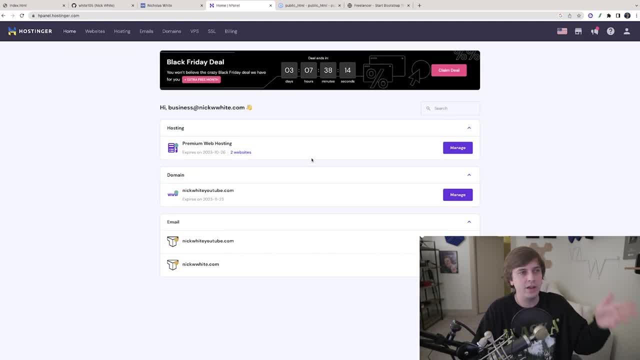 which is pretty awesome. and then it's so easy, right? you have the website builder, you have the WordPress or you can code it yourself. you can do all these different types of websites all on Hostinger, because they're that great. now the fourth and final way to build a website, which is pretty funny and I 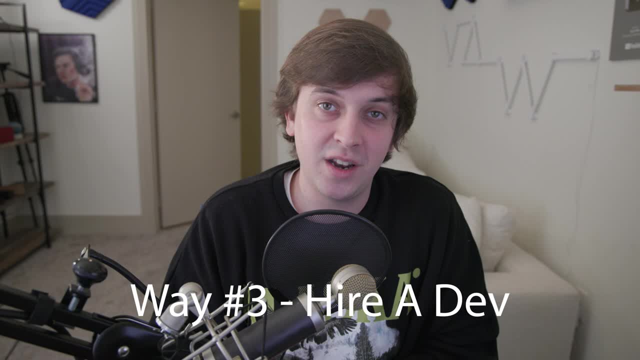 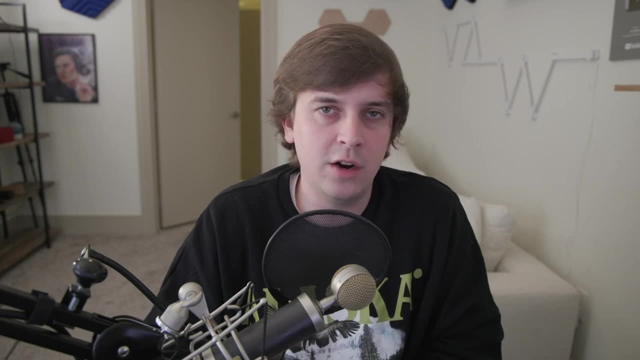 didn't really go over yet in this video is you can hire a developer. now, this is really for when you're on a time crunch and you have extra money. you're gonna want to head over to Fiverr or Upwork and hire someone to build you a simple. 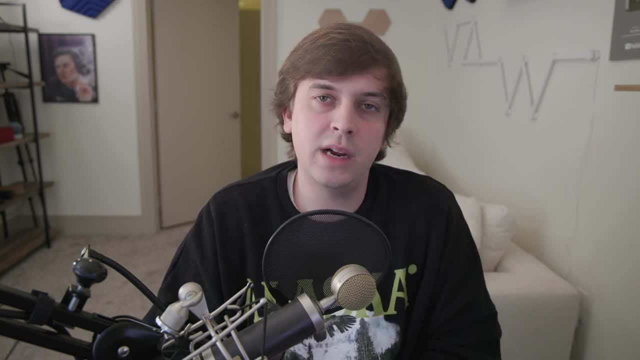 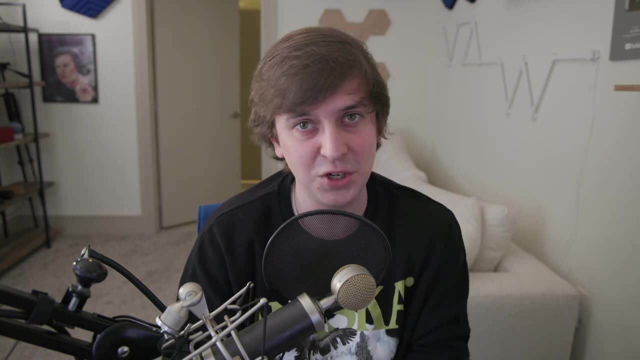 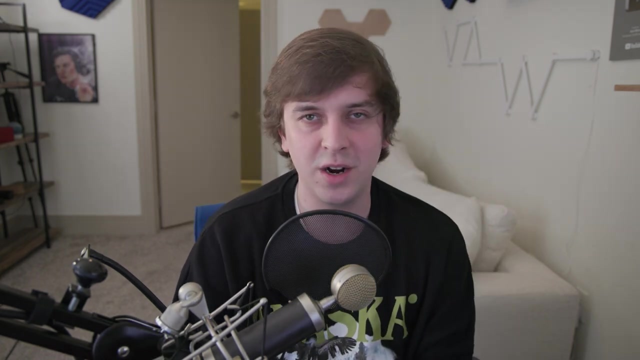 website. prices will range based on the quality that you expect and the complications behind the website. but I'd imagine most of you guys are programmers and you are going to take the initiative to build your own website, not only because you can but because it's fun. but if you do, on a pirate developer to build. 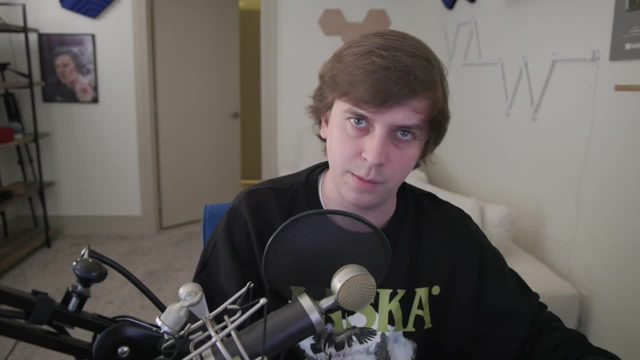 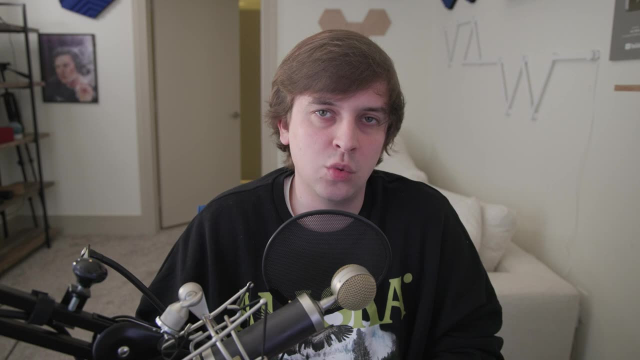 your website from a site like Fiverr, Upwork. those are the two websites I'd recommend using, but, in all seriousness, I used to be a freelance developer, so if you are gonna hire a developer to build your website, please be conscious of how much work people have to put in to actually build these sites. it's very difficult, especially if your website has a ton of functionality. so I would probably just let you know that the more functionality function the website has, like complicated things that it needs to do, the more difficult for developers. so be conscious of that: either pay them more or be aware that it's going to take. 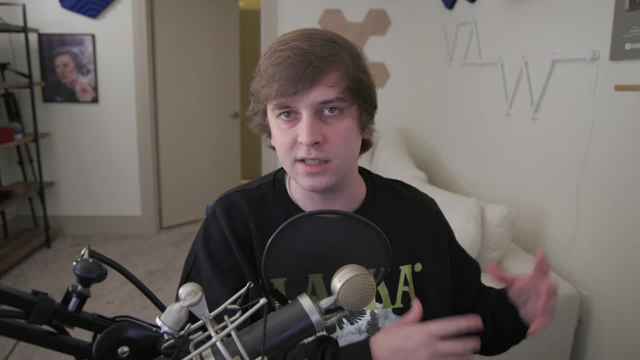 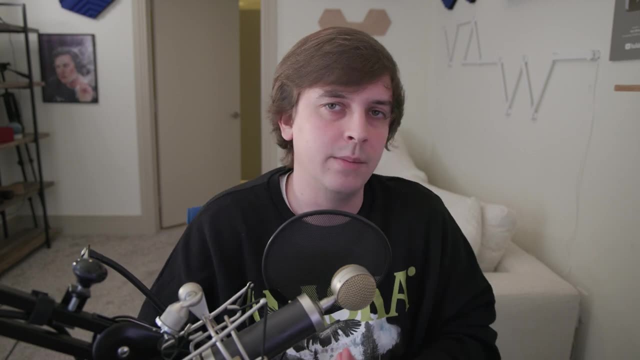 a long time. but vice versa, if the website is super simple, like it's static and it doesn't really do a lot of work, I'd recommend selling it to a developer like That's the one. I would recommend anything, but you just want it to look good, that's probably not going to be as difficult, or? 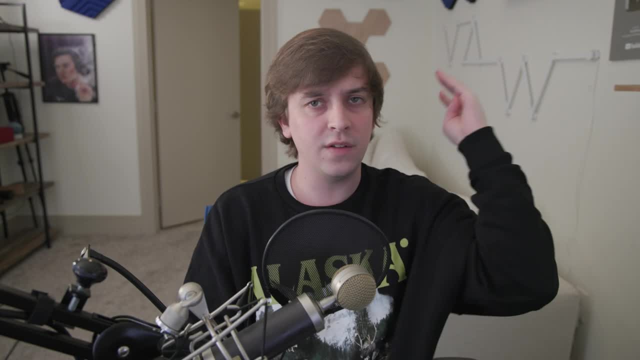 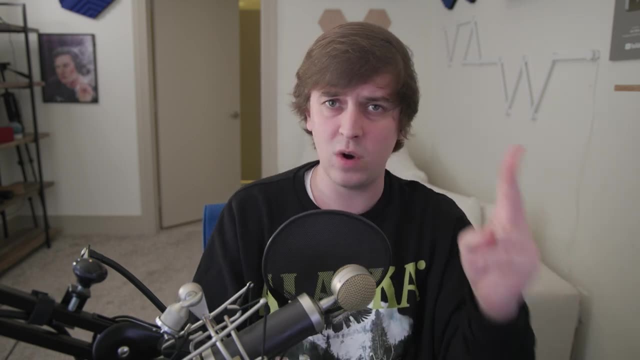 time consuming, So don't get ripped off. So those are the four ways to make a website. If you don't know how to code, use a website builder. If you have a really large content based website, then use CMS. If you want full control over the design and functionality of your website, then you're 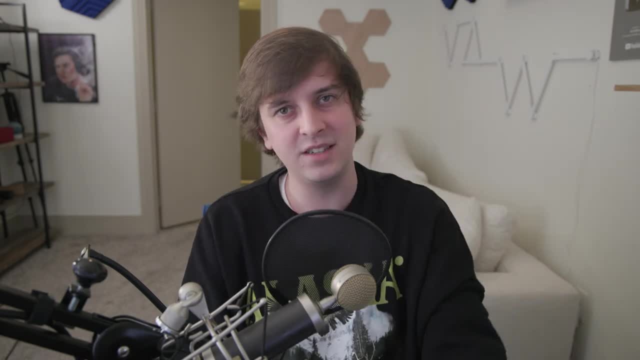 going to want to code it from scratch. And if you have a ton of money, if you have a budget and you don't feel like coding it, then go ahead and hire someone from Fiverr or Upwork. But if you're a 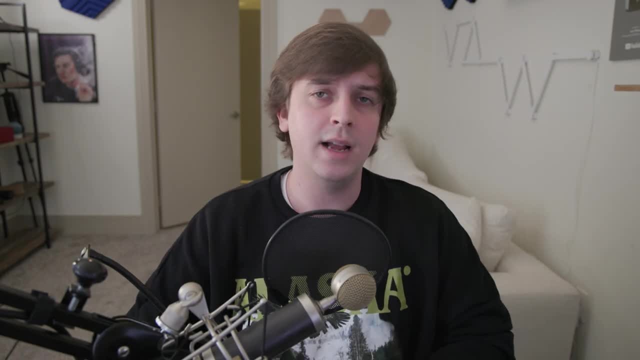 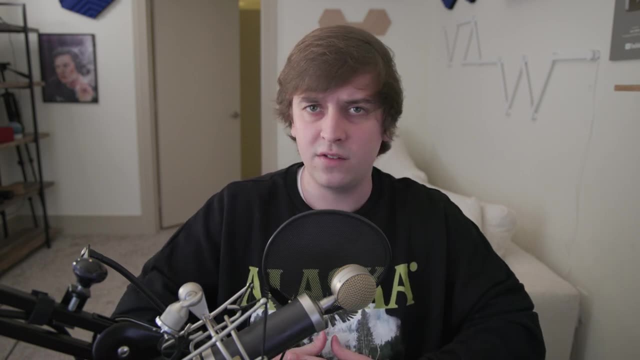 programmer- and you probably are because you're watching this channel- I highly recommend coding the website yourself or doing some CMS because you can get good experience. You could showcase that you know what you're doing and it's really important when it comes to applying for jobs. So 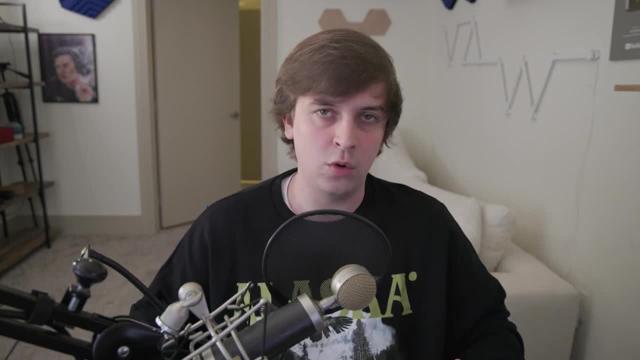 if you're a programmer, go build your website right now. Get your portfolio up. Put some stuff you've done in the past. Throw your resume up there. So, if you're a programmer, go build your website right now. Put some stuff you've done in the past. 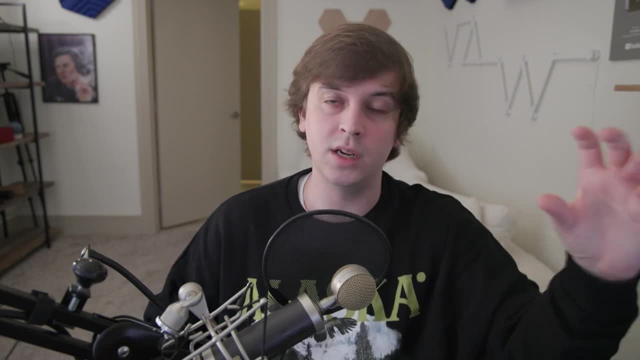 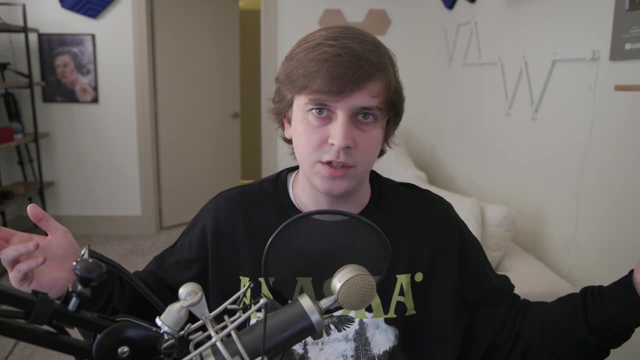 some projects you've done. You could actually embed the projects into the website. if you spend some time and then throw it up on Hostinger, You get the free domain, you get the email- two bucks a month, I mean. I purchase all of this stuff. 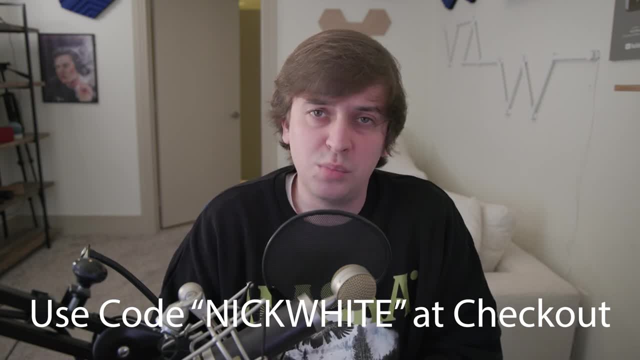 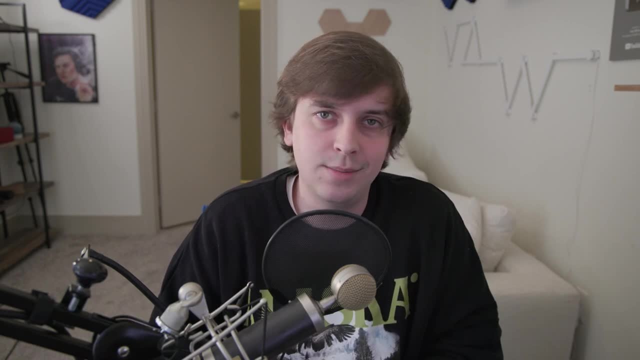 I use Hostinger, So it's really great. It's a Black Friday sale right now. Definitely check it out. I thank Hostinger for sponsoring this video. I hope you guys can build your websites. Please drop some links in my Discord when you're done.